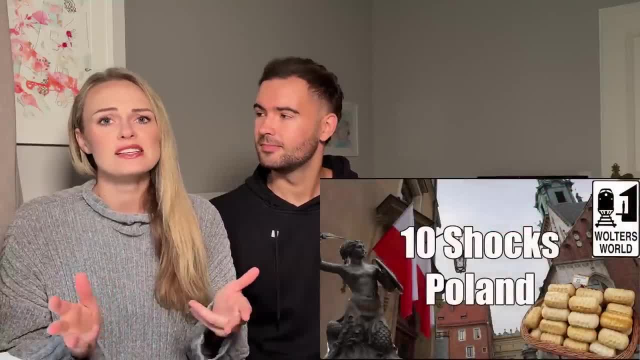 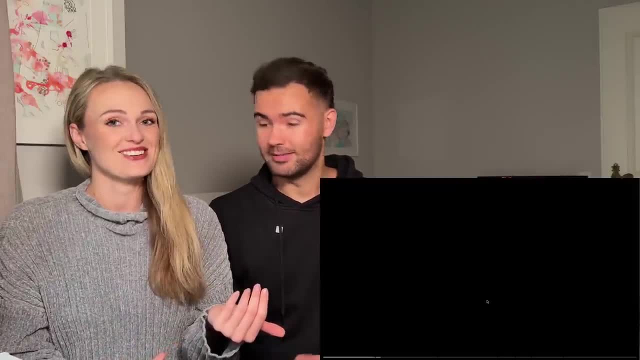 things that we don't know. but actually, every time when I say that we see something that we didn't know. So what do you think? Shall we get into it Straight into the video? Let's do it. Hey there, fellow travelers, Mark here with Wolters World, and today we're in the main square here in Krakow. 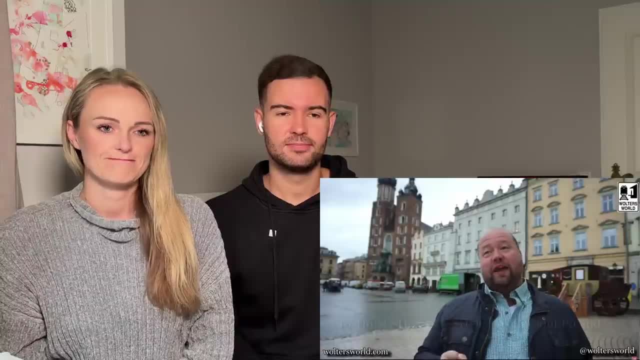 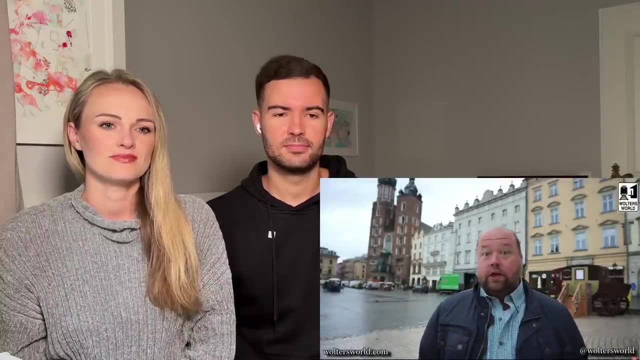 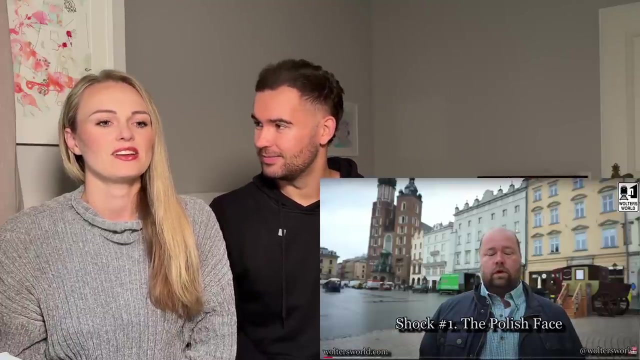 Poland, Beautiful city, definitely worth checking out. and today what we have for you are the 10 things that shock tourists when they come here to Poland, and the first thing that shocks people when they come to Poland is the Polish face. I think I'd do well there, because 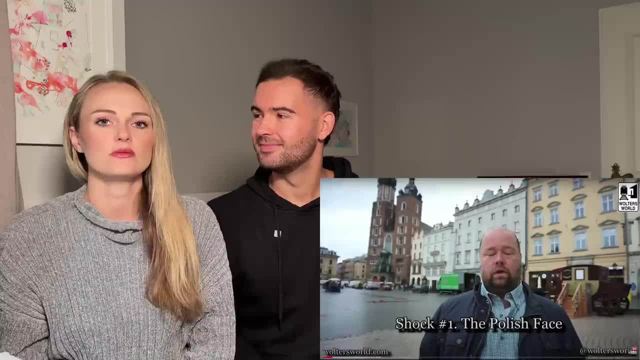 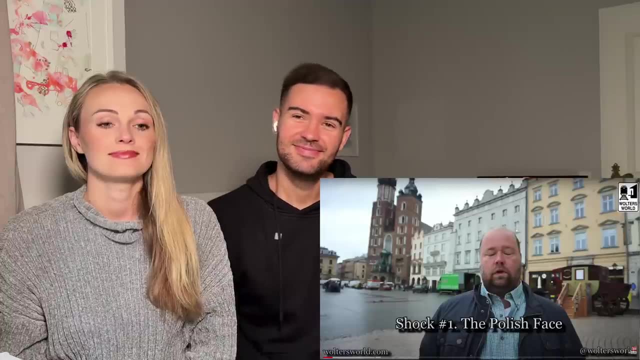 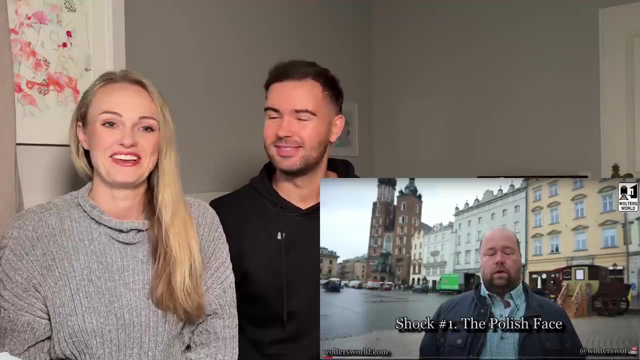 I've heard a lot of times my like natural face, like this one. it looks angry, But a lot of you guys also think that Sinead is Polish. But I'm not angry, it's just my face. I think maybe your ancestors were from Poland. Probably- You never know- You might have had a Polish surname. that. 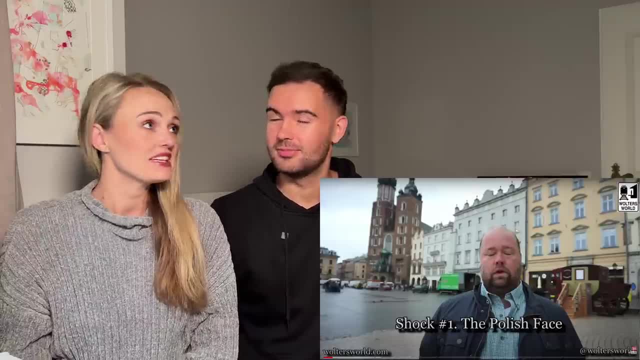 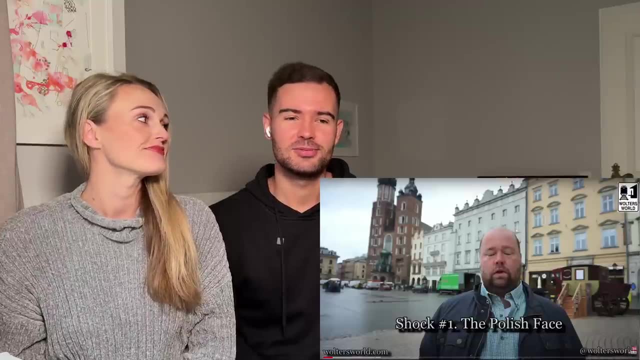 could have changed when your forefathers moved to South Africa. Yeah, you'll never know. We're actually both from European descent, But we don't know. But we don't know the roots. We should probably try and track it at some point, I think so, To see where we came from. Maybe you. 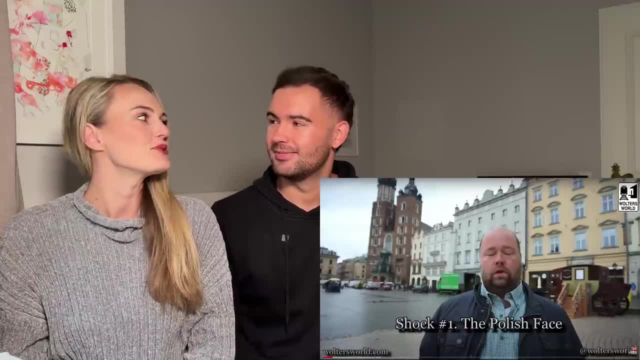 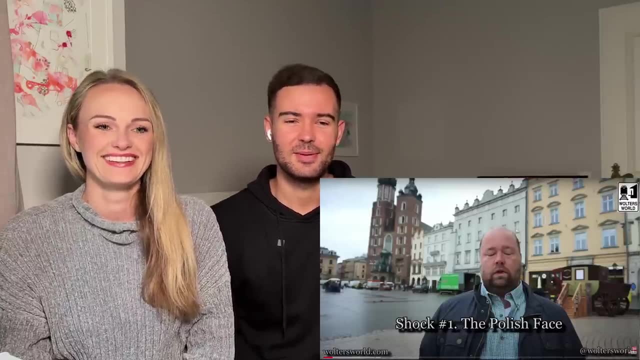 never know. Blue eyed, blonde hair. There's a lot of places that have blue eyes and blonde hair. I don't know. What are you guys thinking? Do you think she's Polish or not? Okay, let's go. But the face, though, to be honest, like that's a lot of Germans also like that. 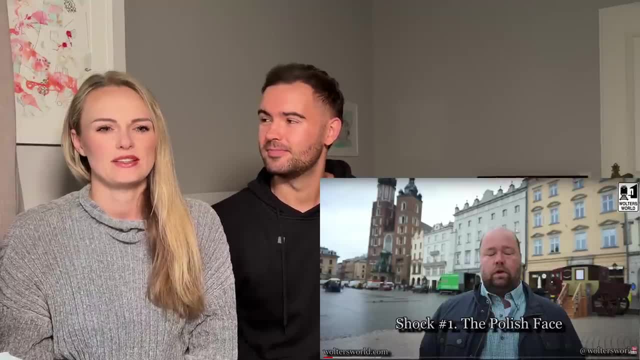 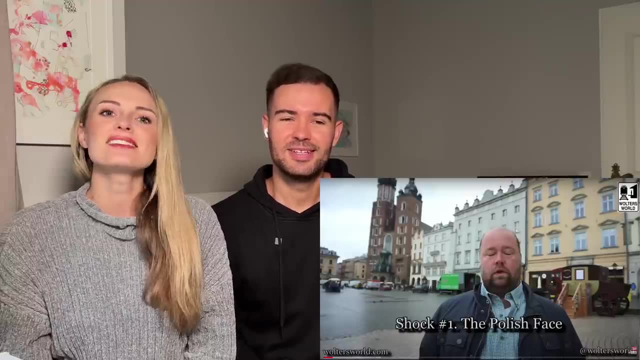 This resting, aggressive face. Maybe it's a bit worse in the wintertime, when you don't see the sun for a long time, I think in the summertime. why would you have such a face, Unless it's your natural, like, normal face, like mine, I have a normal face that looks angry. 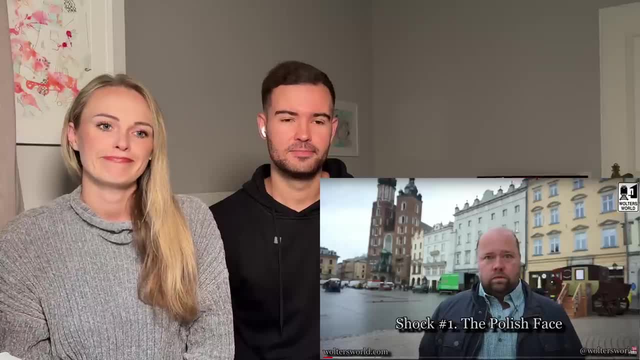 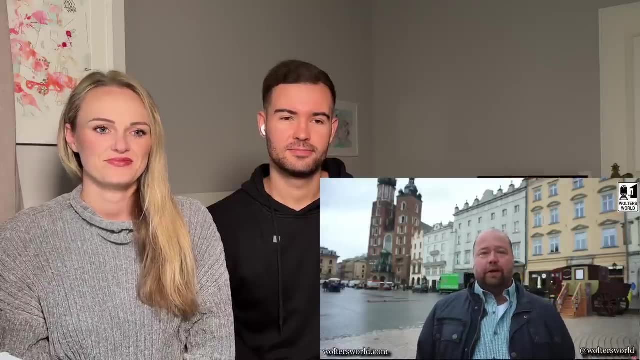 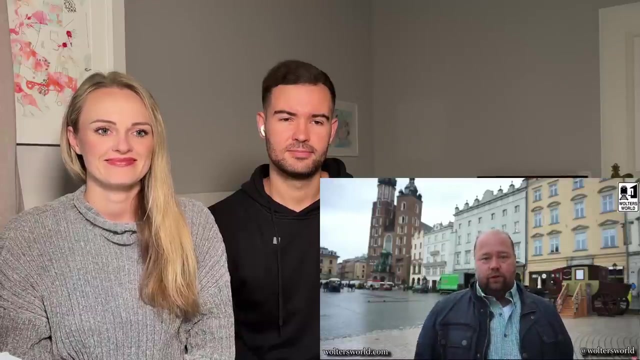 but I'm not Yep. So the Polish face, the Polish look. When you come here, you'll notice that people walk around like this: Just there's no emotions, It's not happy, It's not sad, It's just neutral. And it's funny because you see it anywhere within the train station. You're going out to eat. 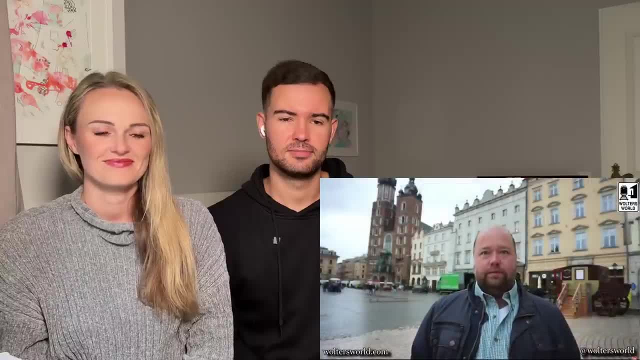 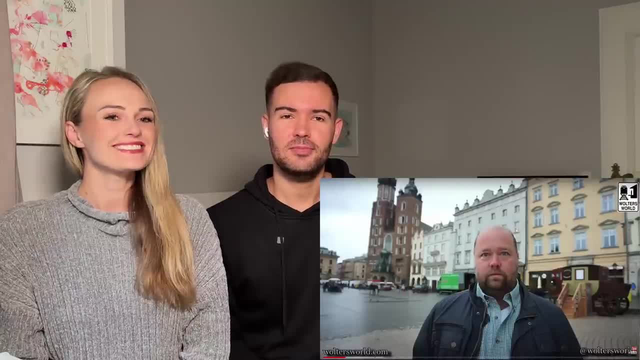 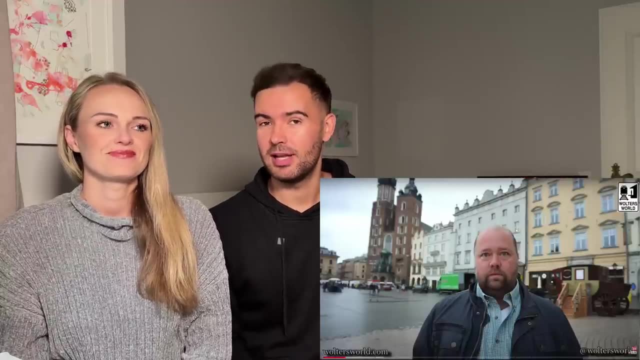 What are you supposed to do? Are you supposed to be like the entire time? If any of you have ever been to South Africa, you will know that it's a very vibrant place. People are always smiling, No matter what state you are in, where you come from. 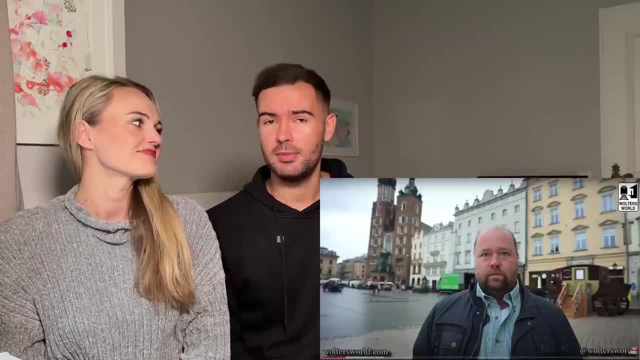 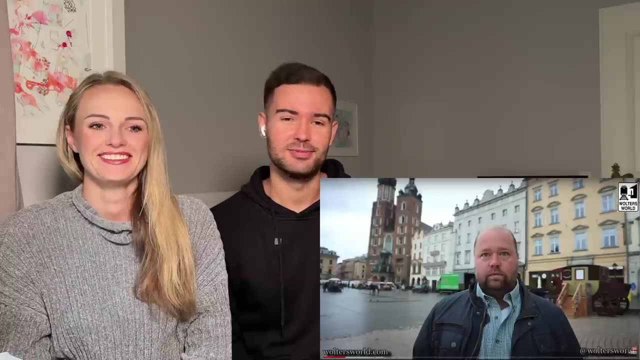 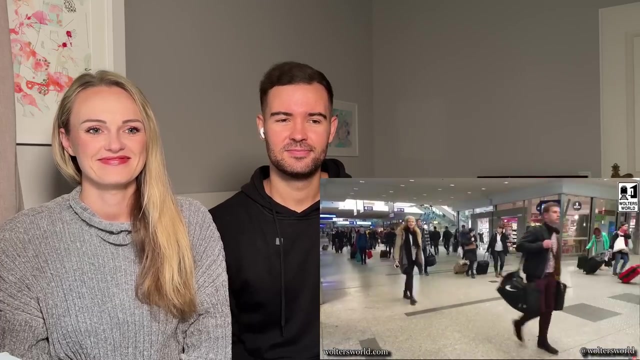 a lot of South Africans are vibrant. a lot of people i meet in europe prefer to use africa as being bright and colorful and vibrant, because people are very friendly and nice and i think it's just europe in general and you're like: wait a minute, can't you be happy or sad or something? no, they have this like dead-on look. 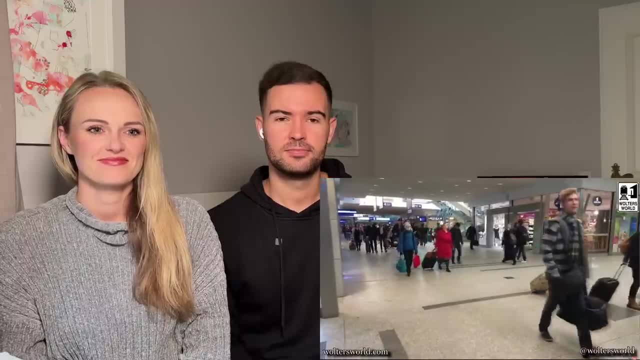 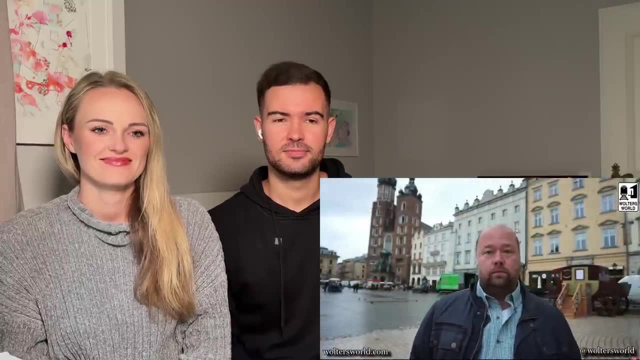 which works really well, because you'll see, the women here are gorgeous, okay, and when you see them walking, oh, they're just preparing for their supermodel career, because when you're on the cat walk you don't show any emotion. so they actually works really well. but it's kind of funny how the 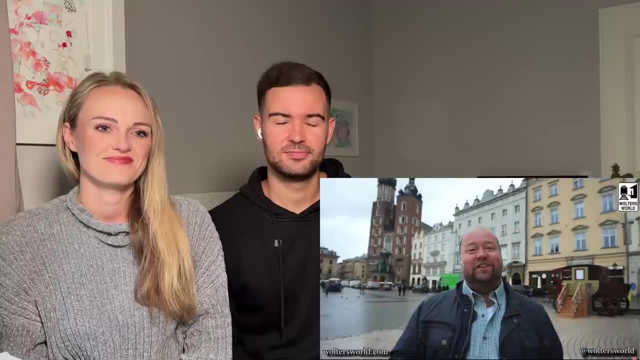 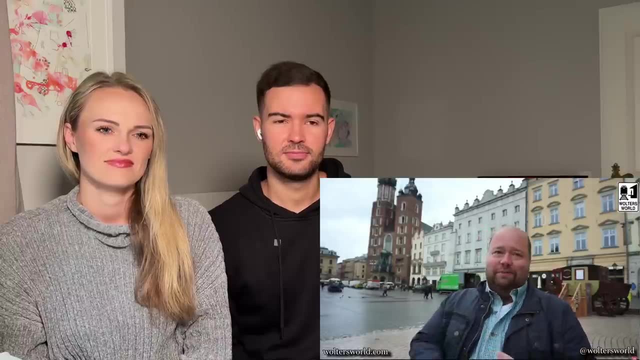 people you know you do have this. look, and that's the first thing that shocks people also, kind of going along with the people, you might be shocked that look, the polls are not like the jokes you heard as a kid. they're not dumb, they're not alcoholic stuff like that. you don't have that. 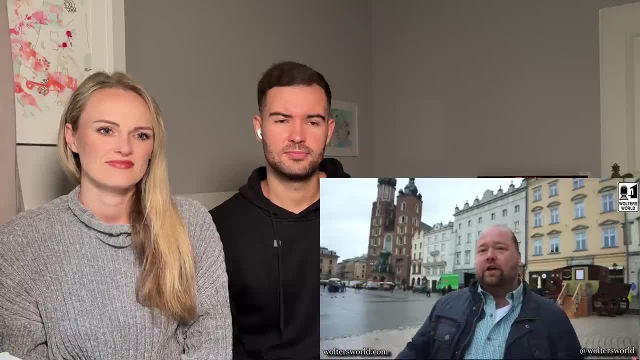 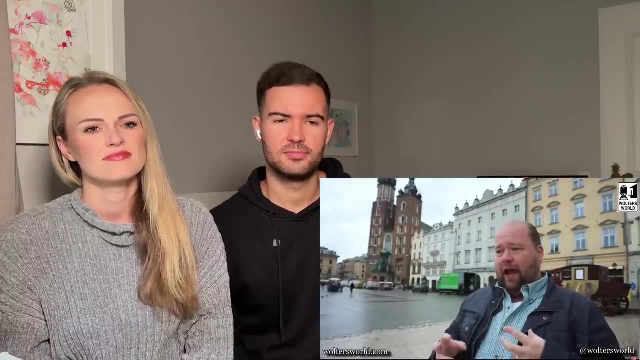 i mean, yes, there are, but that's everywhere. it's not more or less than you get in other countries. so that also kind of shocks the people that come here, because i'm used to all those polish jokes where: what is it for polish people and how do they? 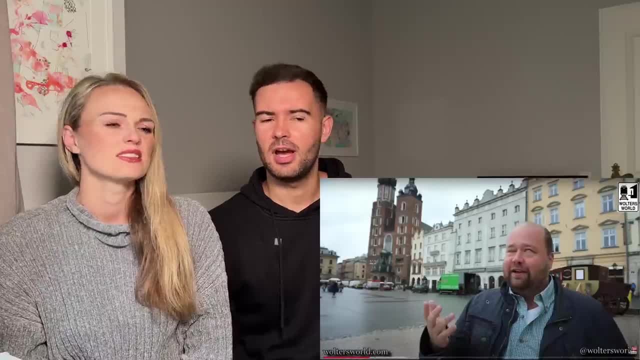 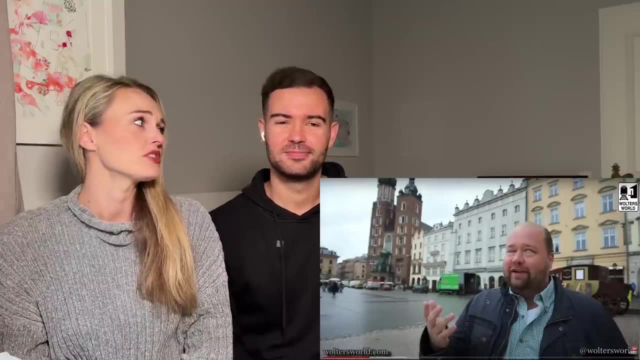 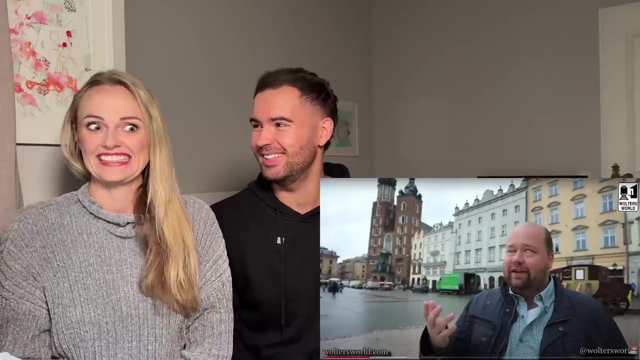 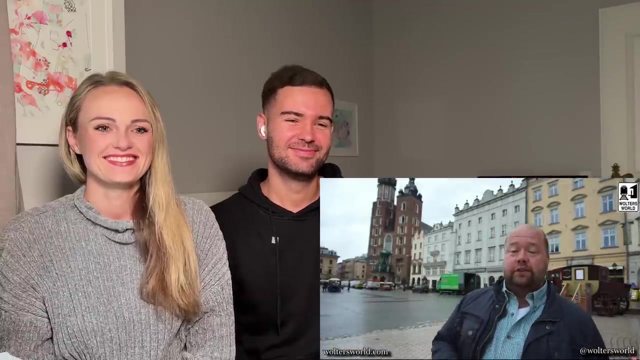 you know, move the bed or something. i never thought polish people were dumb. i've never heard a polish joke either. it's a weird frame that breezed it on right. americans are weird. yeah, you don't have that here. the second thing that'll shock you when you come here also deals with the 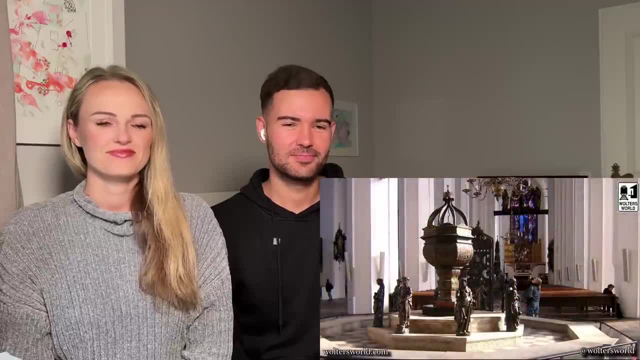 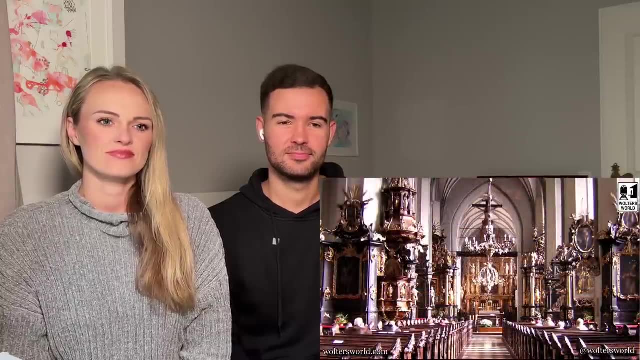 polish people are, how catholic and how religious the people are. i mean, i remember going to the church and i was like, oh my god, i'm going to the church, and i'm going to the church and i'm going on the buses and lublin, and these like punk rock guys are on the in there and and they go by a. 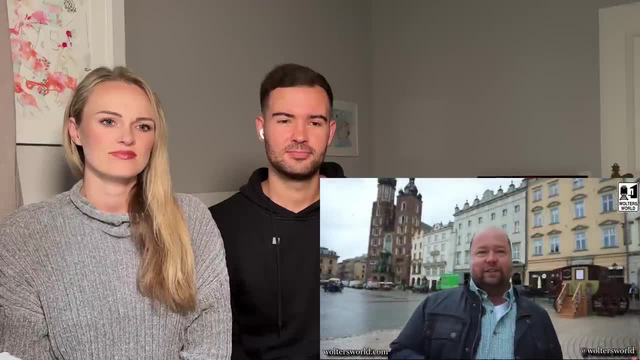 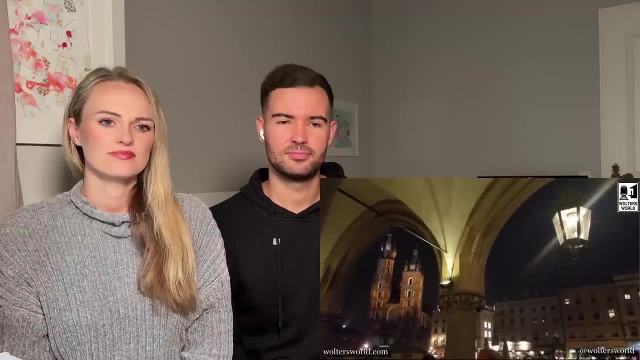 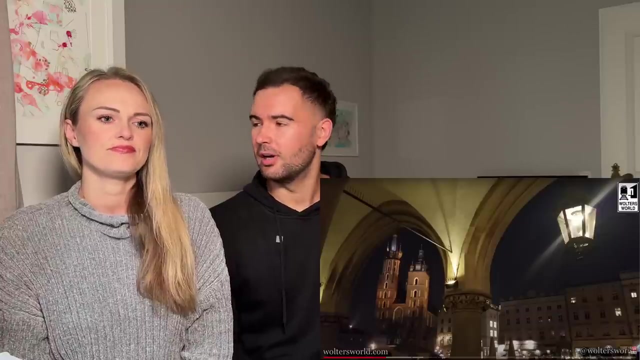 church and they all do the sign of the cross. i'm like whoa, i didn't expect that. people here in poland are very religious- and the churches- this is saint mary's. honestly, the first time i walked in there 20 years ago, i would just draw a drop. wow, the blue, a lot of. also, i want to say europe has. 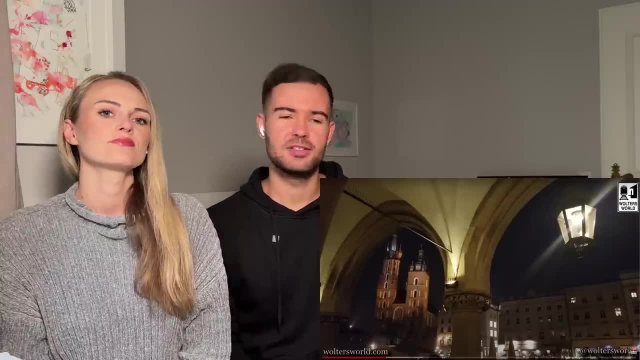 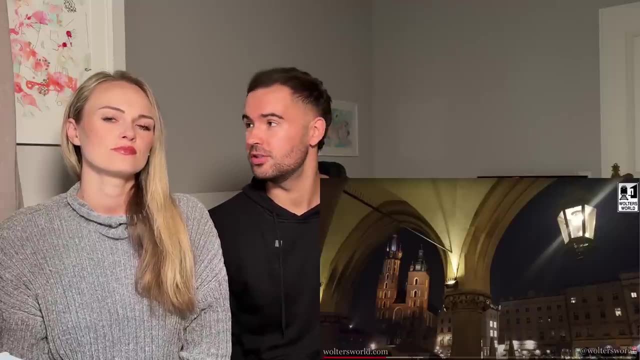 got a lot of church, a lot of catholic, christian, jewish ancestry, which is very nice. um beautiful buildings, some of the most beautiful buildings, i think, in any city- or the churches- yeah, you don't see that type of architecture nowadays being built um. i always find it like 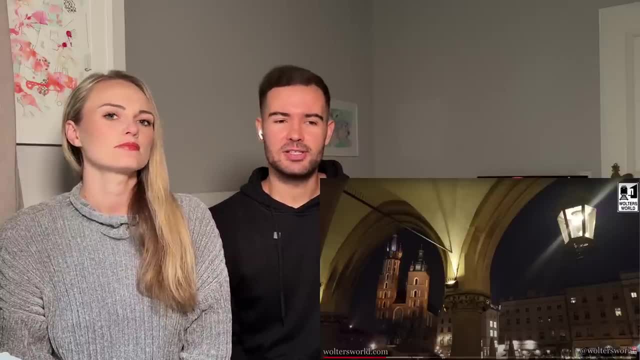 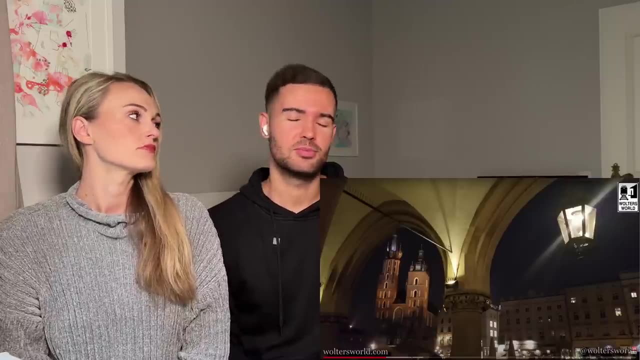 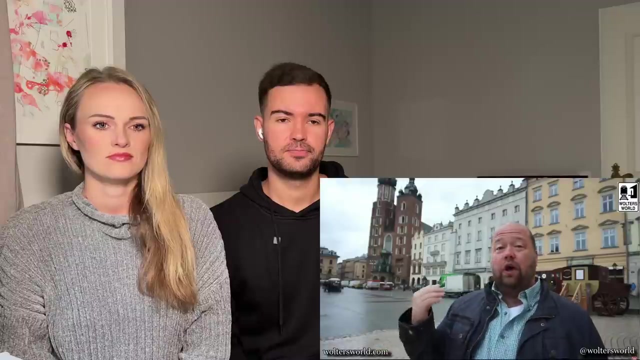 stunning to just look at and just just look at the statues inside. uh, so much history and the fact that a lot of those survived so many wars. it's pretty cool to see the all blue altar in the blue ceiling and everything. it's just amazing. and the churches around the country are gorgeous and they're. 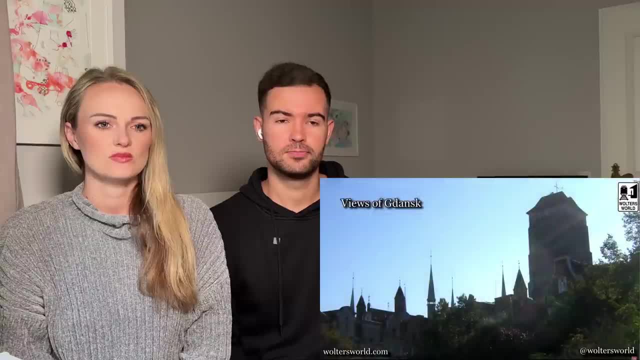 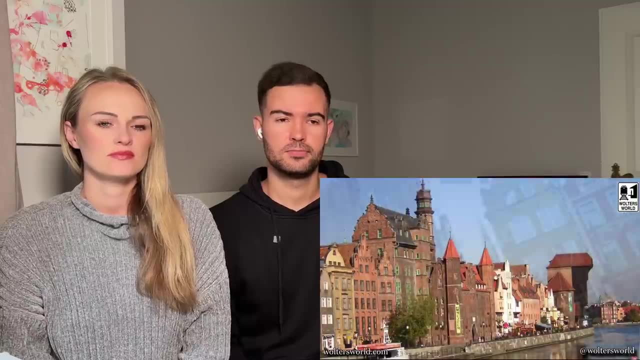 actually building more churches here. you know other countries. they're turning churches into apartments and hotels and bars. here people still go to church, they still do believe and you do have a very religious, conservative feel when the people are here, which is kind of a different thing, and 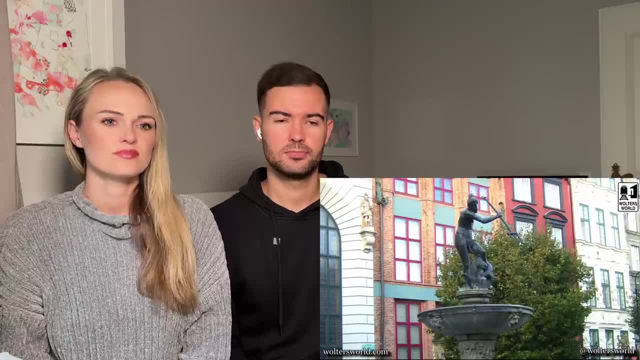 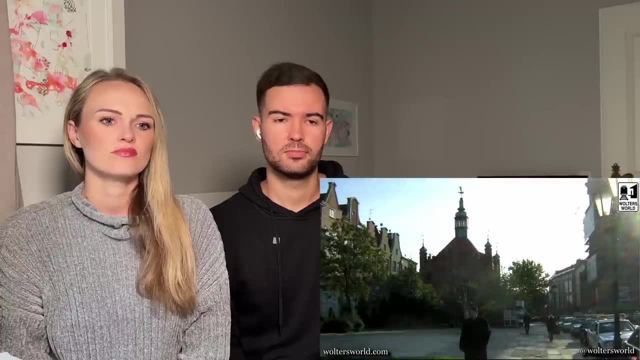 you go and when you go in the churches- that's the real thing about it- you really see the beauty of the churches, the ones that haven't been destroyed during the war, um that may they've been rebuilt, but like here and other ones, you really go in and just see the majestic beauty of the churches here. 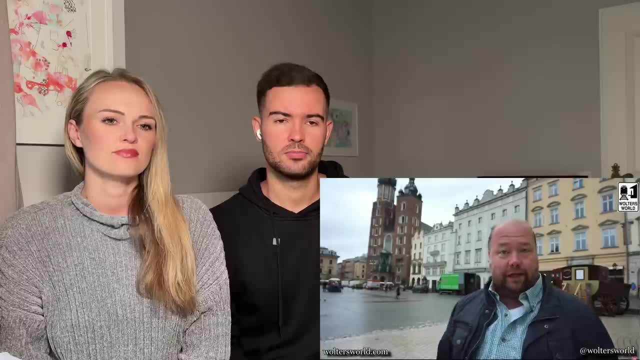 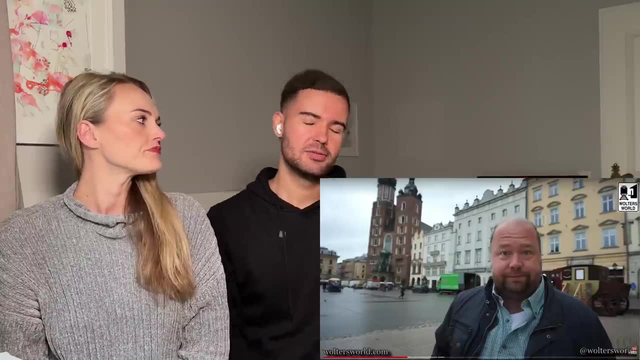 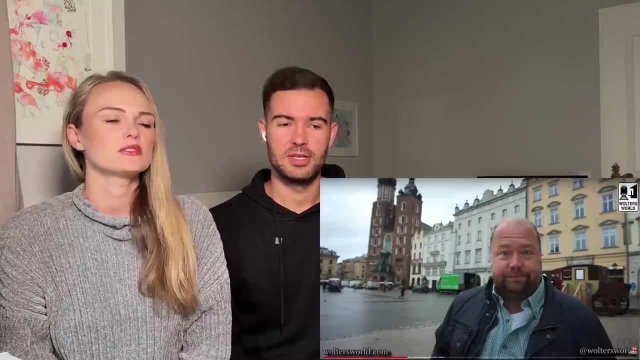 and i think that's what's so interesting about it- is that you don't have to go into the churches, don't just go- oh it's another church, go in and check it out. i like that fact, like i like that they are religious and me too it's. it's nice to see that. i think it installs a lot of morals in. 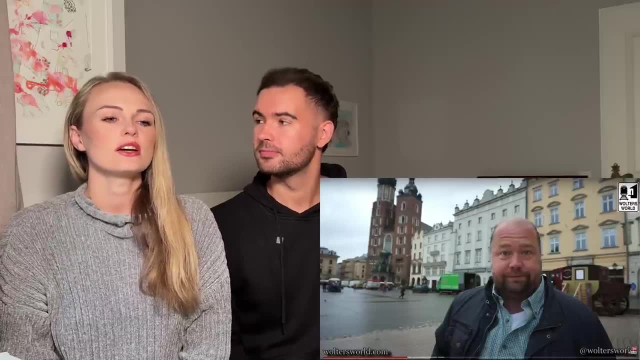 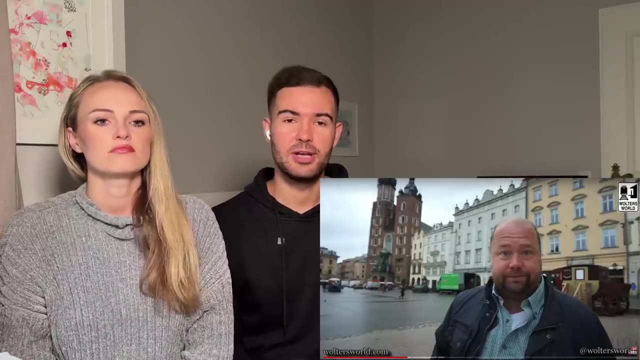 in people and you know, when you see someone live according to those morals, you can actually see it in the country, the people, the, the safety that you feel they're that kind of leads into. the third thing that'll shock you when you come to poland is how much 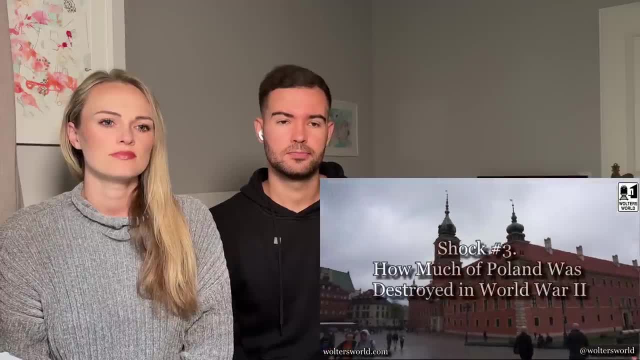 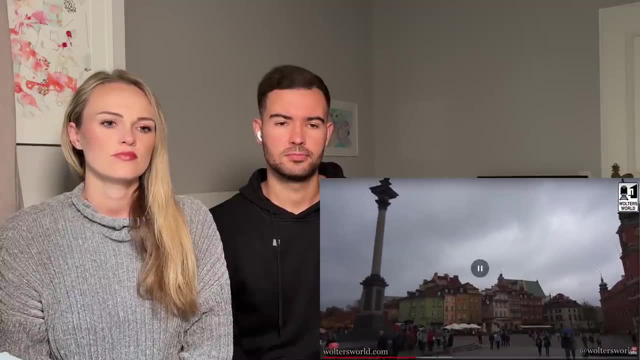 poland was destroyed during the second world war. i mean, krakow was lucky. it didn't really get destroyed during the war, but a lot of the other cities were just leveled, for example warsaw. when you go there, you'll go. we saw that, or we didn't see it, but we've seen it in videos- uh, warsaw being 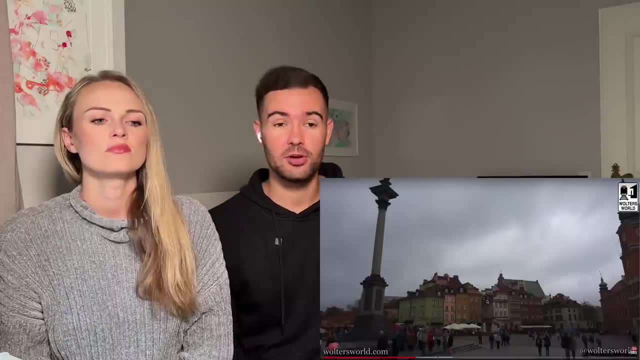 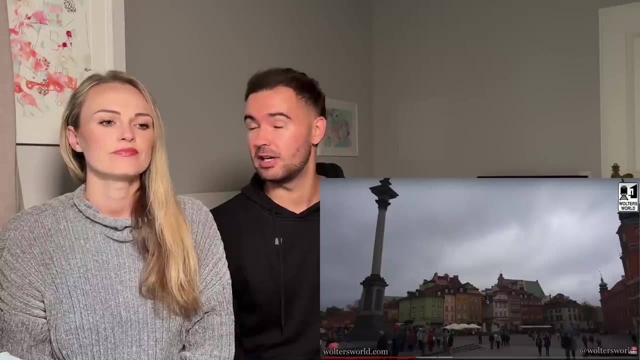 like 90 demolished during the war, but a lot of the cities um all over poland and have just been completely annihilated in the war. and i think that's what's so interesting about poland is that poland has a lot of history, and a lot of history in the 40s, 1940s, and a lot of work was done to get 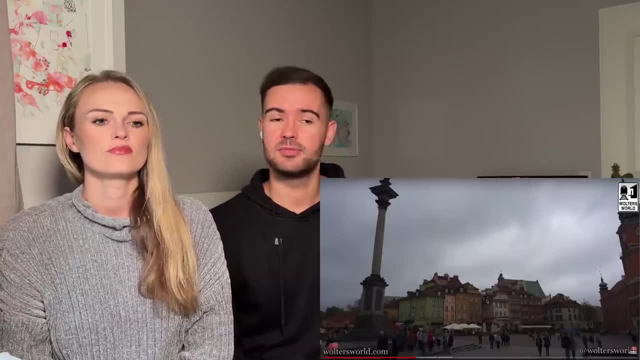 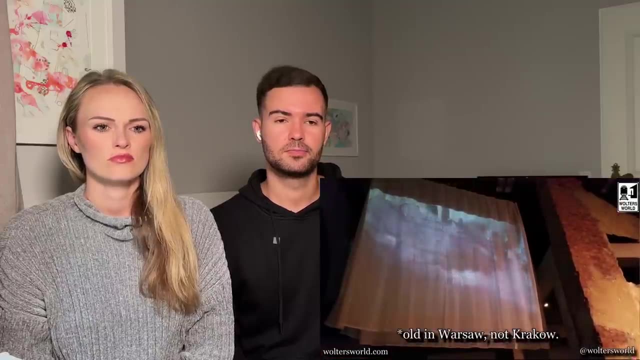 them to where they are today, to kind of look the same same feel. go see the uprising museum and realize that everything old in krakow is actually younger than probably your dad, because they had to rebuild it all after the war because it got leveled by the nazis, and you'll. 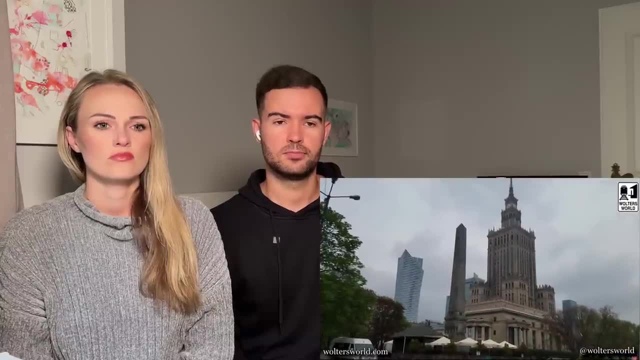 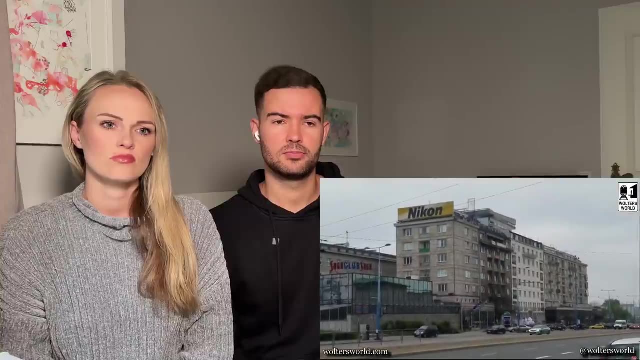 see that and you go around. that's why you'll see the communist architecture in the big square: long rectangle buildings and stuff like that. because there was nothing there, it was all destroyed so they had to rebuild. and when you really see the level of destruction throughout the country and 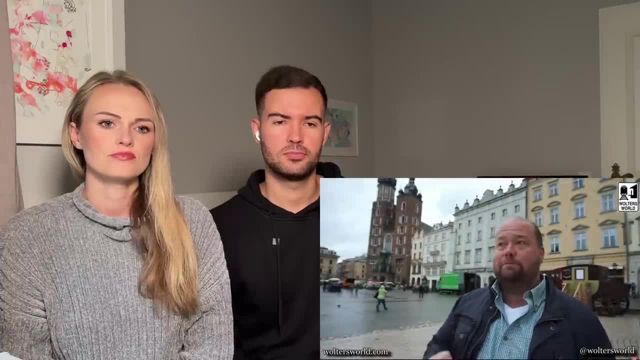 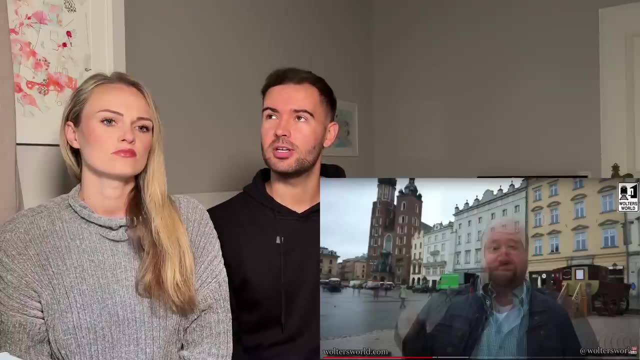 how much they've come back and built new stuff. you'll be very proud of the people, and that's what's really cool about it. now, one thing that i don't like is i don't like the architecture that was built post-world war ii. it was this mess developed. 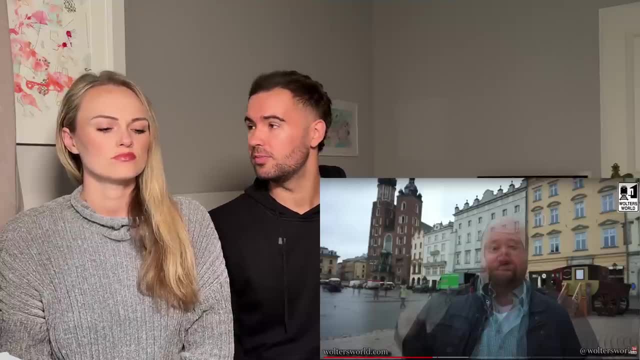 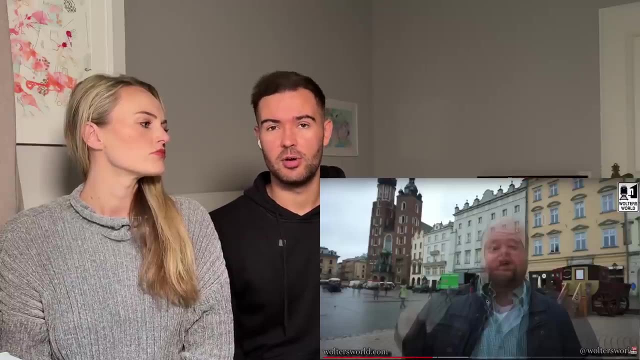 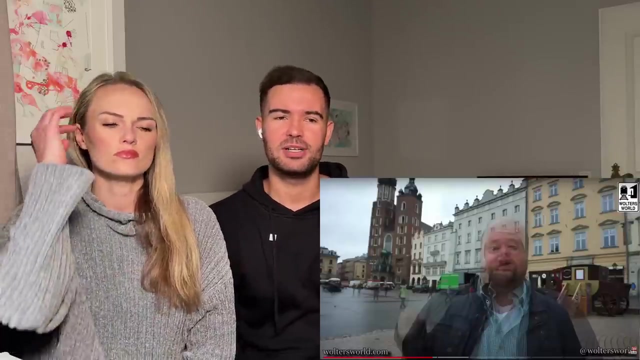 not developed, but mass housing. that went up because of the shortage of places to stay. so even in berlin, which also received a lot of bombings in world war ii, a lot of the buildings were destroyed and then these really ugly looking apartments went up. uh, that just was put up to. 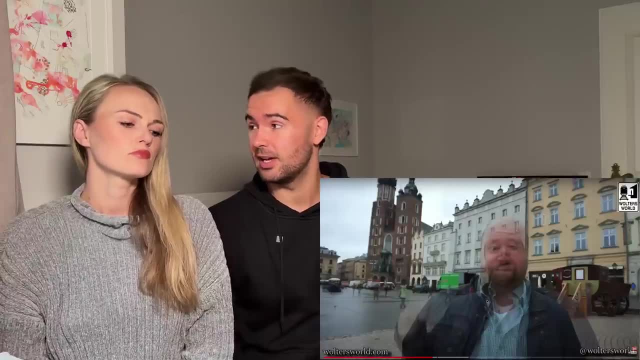 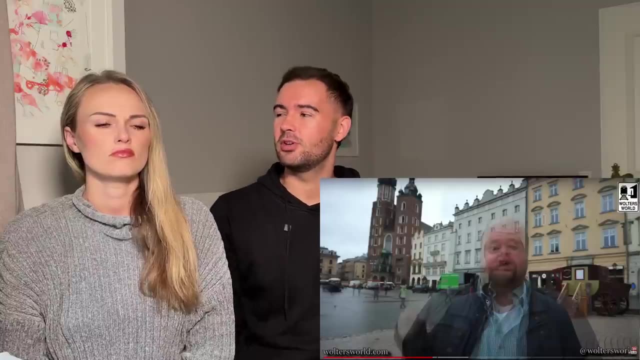 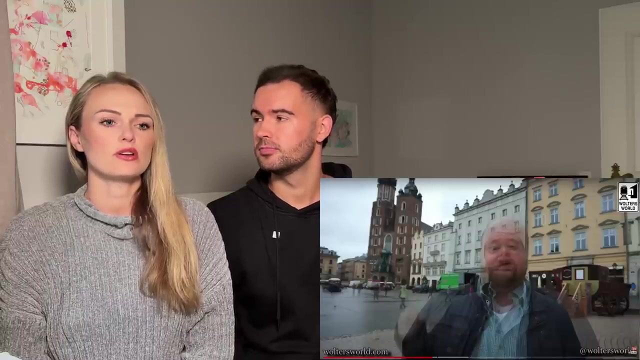 save time and save money and to get people like a place to stay and it's really got this communistic feel to it. but it's not a. it's not as beautiful as the architecture prior to that. yeah, you can clearly see the, the areas where it's pre-war buildings, because those were. it wasn't bomb they really, yes, not. 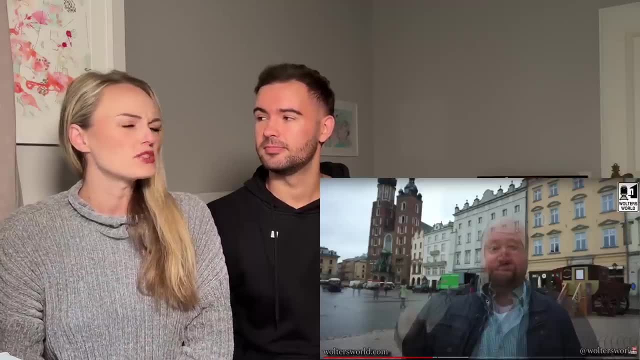 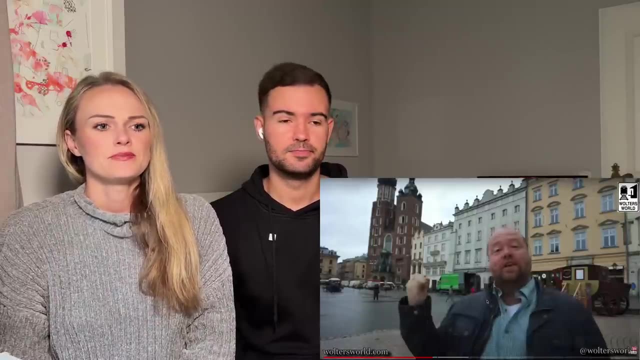 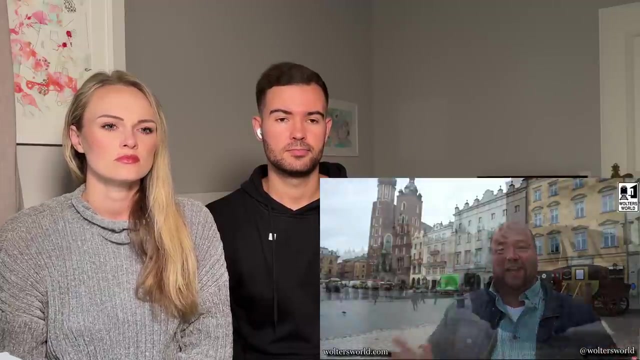 yeah, the ones that weren't bombed. but it's so beautiful, it's majestic though the architecture is is something out of this world. examples now, the fourth thing that's going to shock you when you come to poland is how completely incomprehensible and illegible the polish language 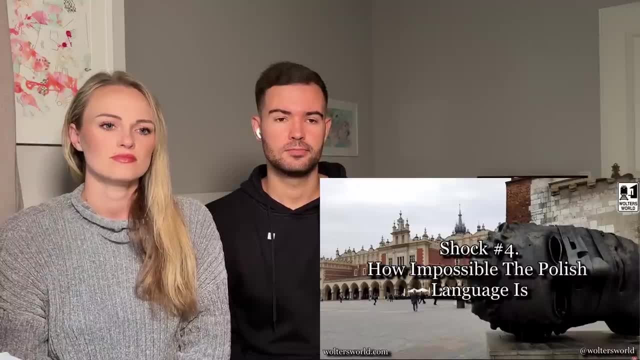 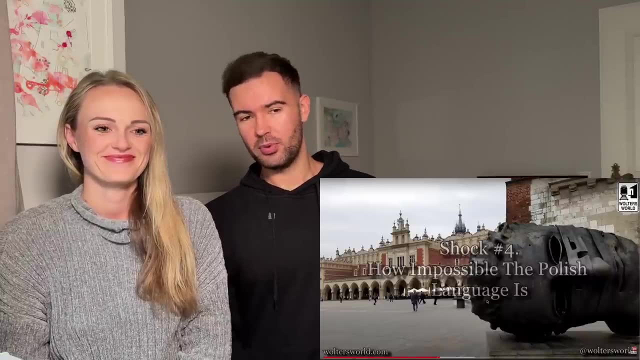 is: look, if you don't speak polish, it's okay, the locals know you don't know how to speak polish- it's okay, the locals know you don't know how to speak polish- it's okay, the locals know you don't speak polish. i feel like the language is also something that is always brought. 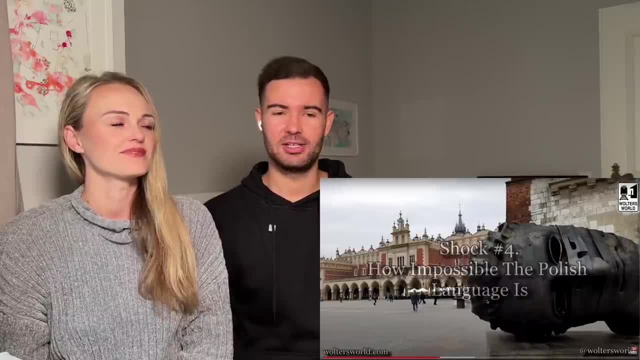 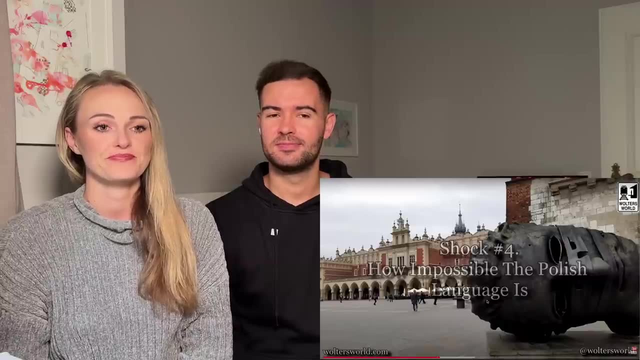 up in some video of how difficult, for how difficult it is, but some people say it's not difficult. that's the weird thing. some people also say german's not difficult. german is very difficult if you don't speak it, if you come from english background, i think. 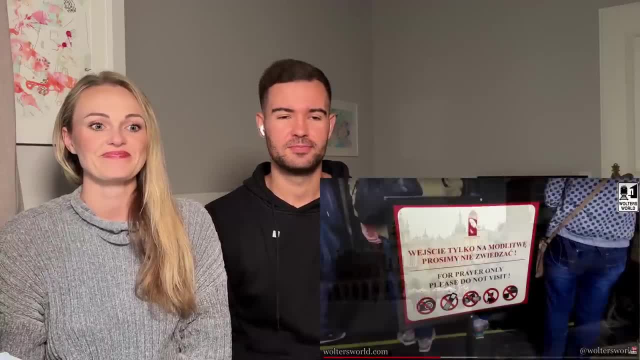 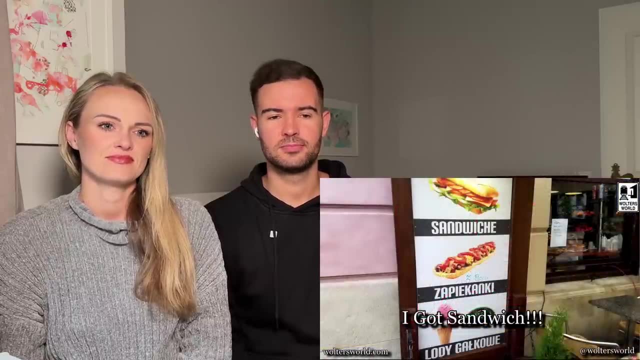 it's difficult. yeah, let's not try to think polish with you, but polish is just one of those languages you're listening. at the train station you're like, yeah, i got nothing. yeah, i got. i don't even know what city i'm going to. it is a very tough language and it's very hard to pronounce. like how do you Say: 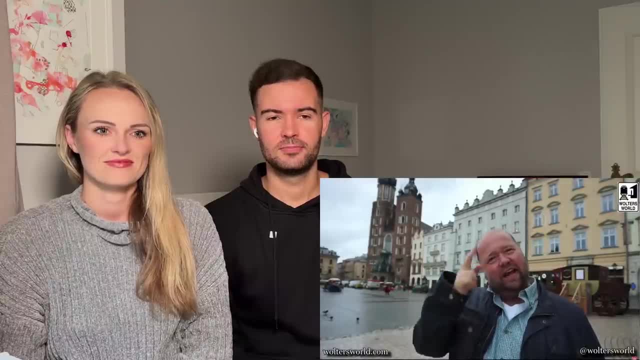 p-r-z in a row and there's like a hat and there's an L with a line through it. is that a t or a w? what is that? you do get pretty confused when you are here and it is kind of shocking that you can't. 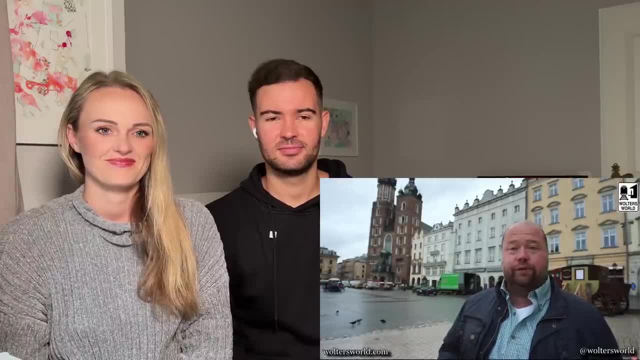 even make out some of the stuff now they are developing better for tourism, so you will have a lot of you know english menus and stuff like that, but it is a really good idea to know some polish before you come. like you have to learn a lot of polish because she's coming from a lot of 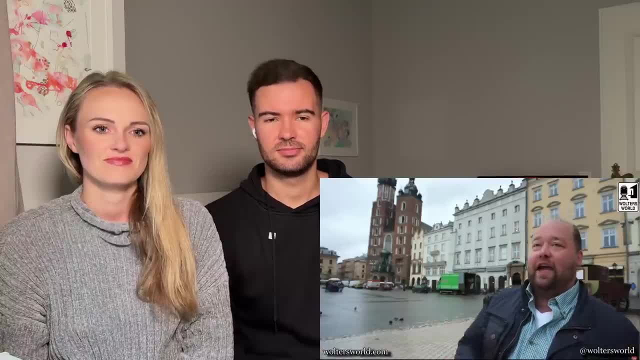 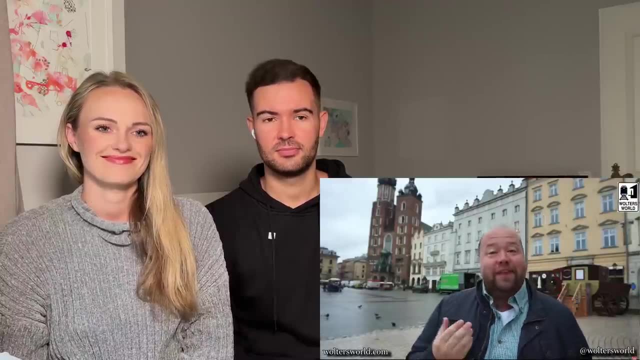 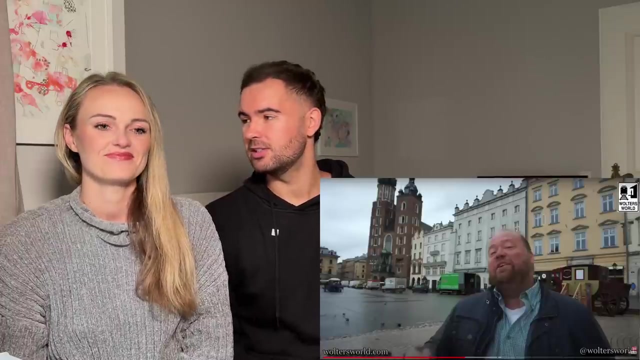 which is like thank you, prosim, is please, things like that, because it really gets those people to go from. you say, oh, you speak polish and they really open up. then okay, i feel like i think the point makes it very difficult. it's just that the fact that the 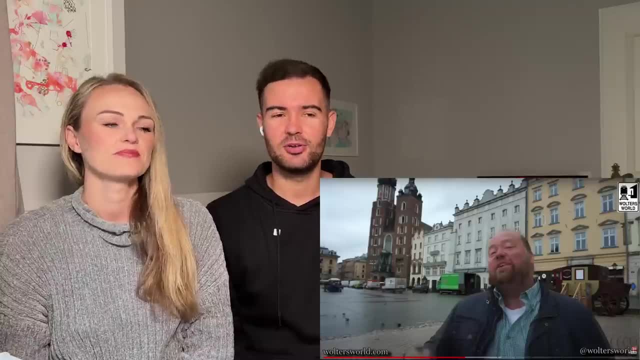 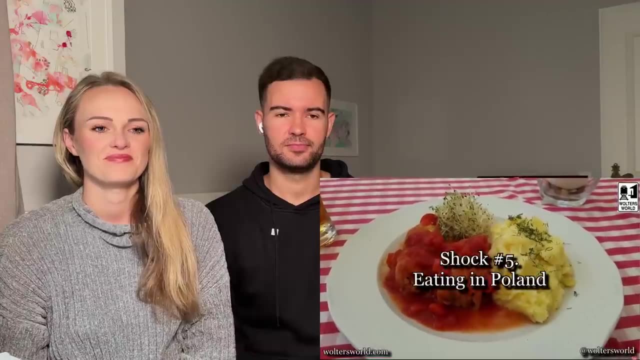 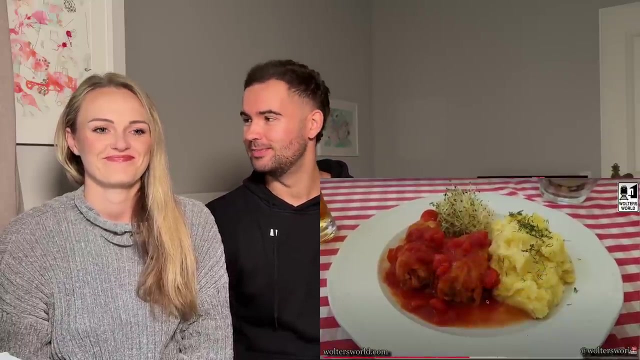 alphabet's not the same, different, yeah, so you don't know how to pronounce, how to pronounce things. the thing that might shock you is your eating experience here. the poles really love their potatoes and their cabbage. yeah, even if it's not on the menu- cabbage, potato meat, but we 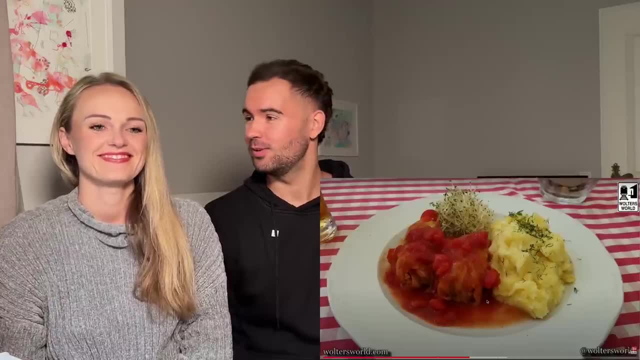 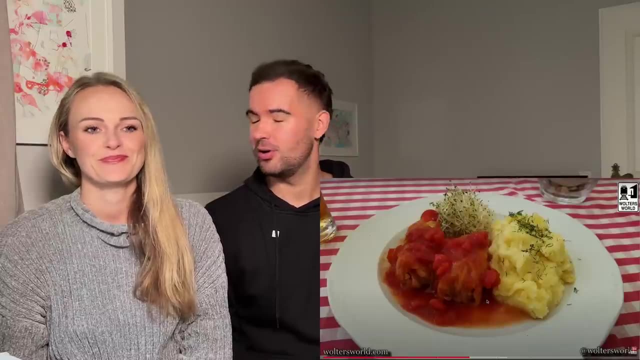 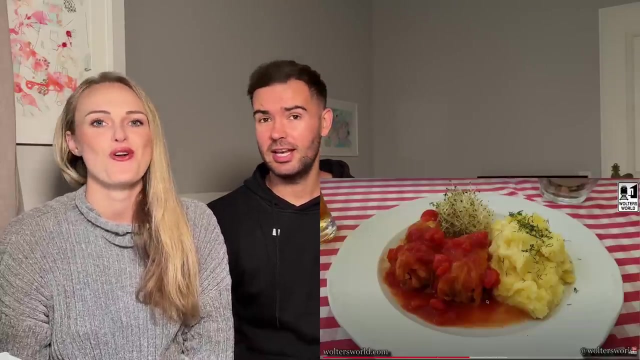 like that too. i love it, even the pierogies that are filled with potato, or pierogies that are filled with like a cabbage. oh, amazing food in poland is something that i am very much, and we keep on saying it. we are definitely going to create one entire media just dedicated to food experience. 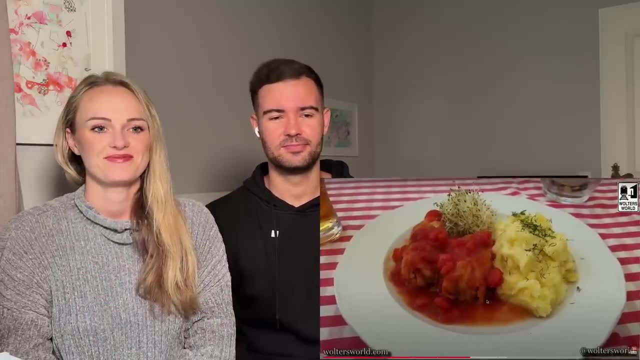 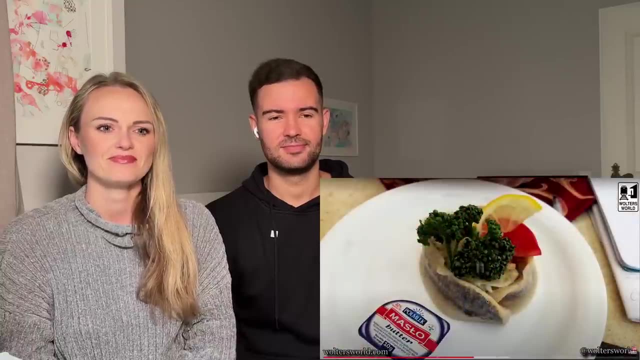 with the food in poland menu, like it may say: oh, it's a cutlet, you nice, it'll come with cabbage and potatoes. oh, i'll have the pork knuckle instead. oh, that's what's in. it doesn't look forward to, though. that's that, that fish. i'm just not a. 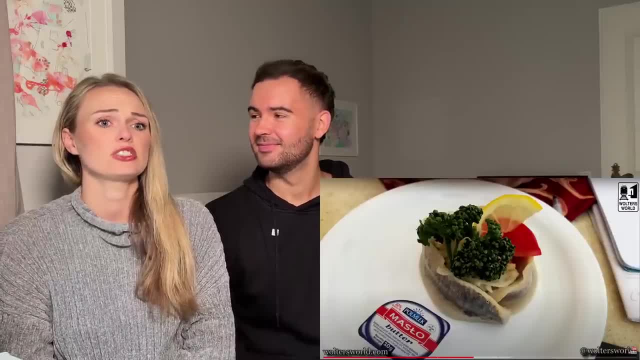 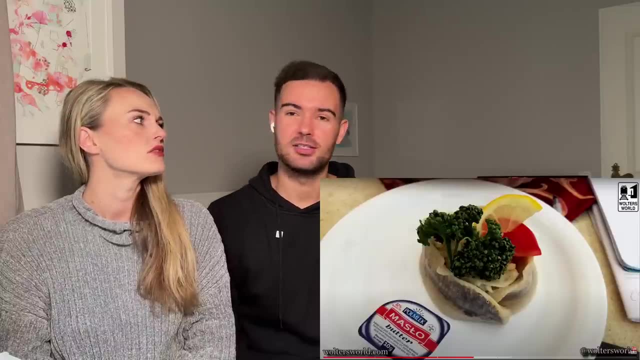 fish person. i think a lot of europeans like fish, like for breakfast and stuff i would. we had it in in session in poland. it was: um, oh, i had it, so i was too scared to try. i just don't like fish, not for breakfast. it was like a- i don't know if that's for men. 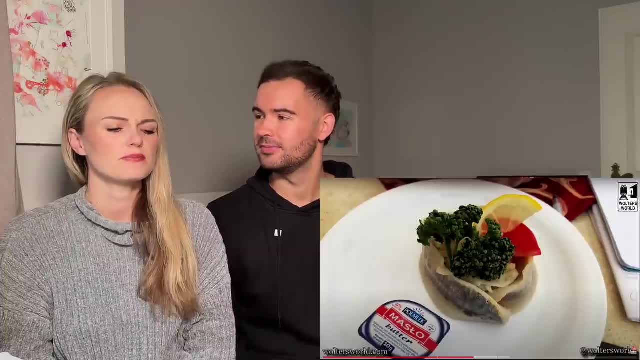 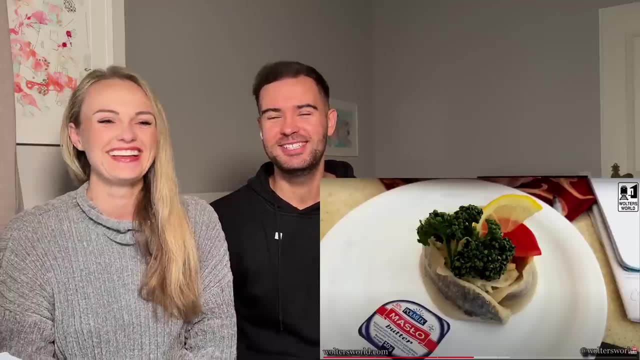 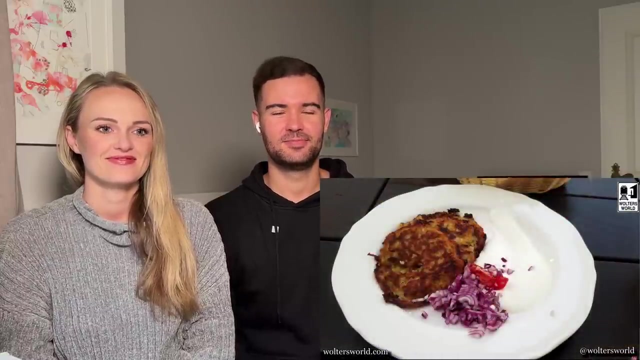 to fish. it's in black brine. um, i only know the africans word soaked. it was no, nope. oh, it comes with pork and cabbage. well, i'll just have the rolls. oh, it's a cabbage roll. okay, you're gonna have a lot of cabbage. you're gonna have a lot of potatoes. 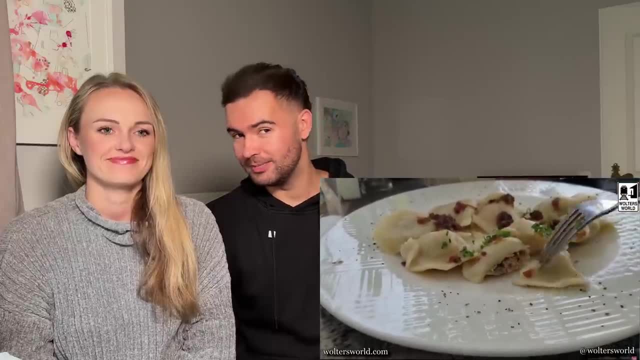 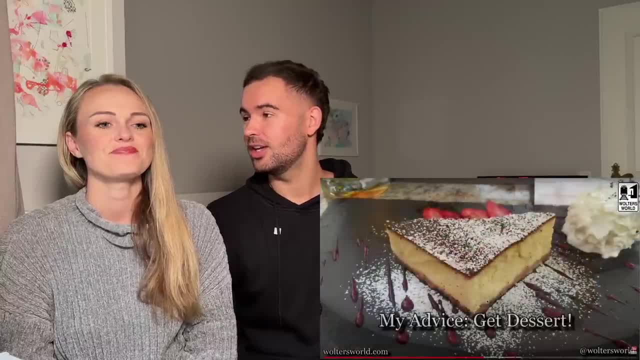 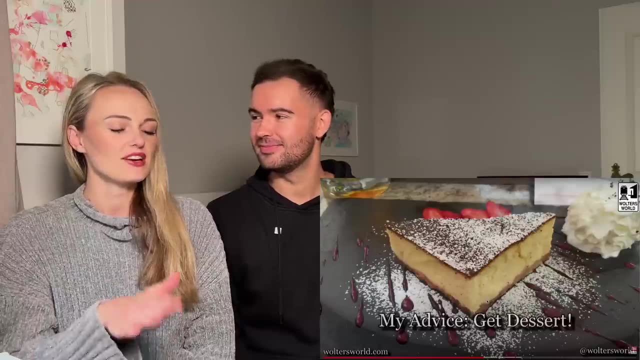 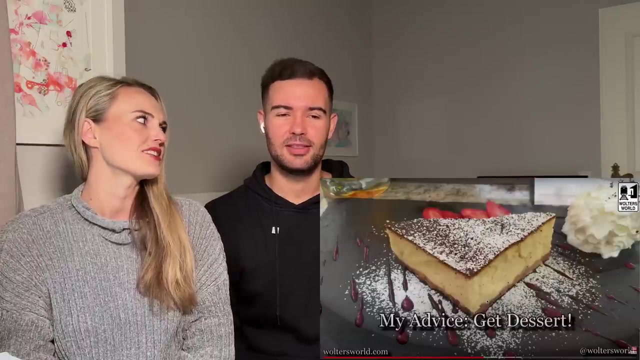 potatoes. but someone said that we can choose how you want your pierogi. you can choose to have it steamed or you can choose to have a deep fried and crunchy. i think they like. they can also like just fried, quickly crunched out. that's what i said. yeah, but not deep fry. i don't know about that. i. 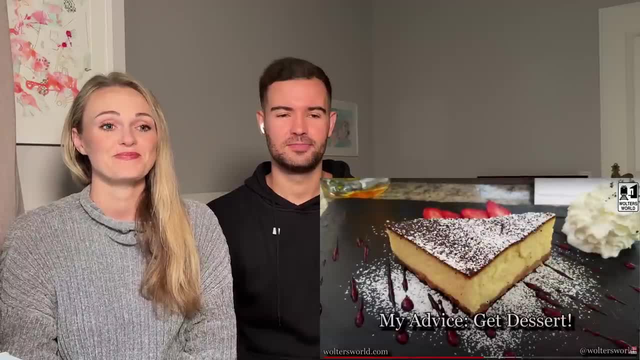 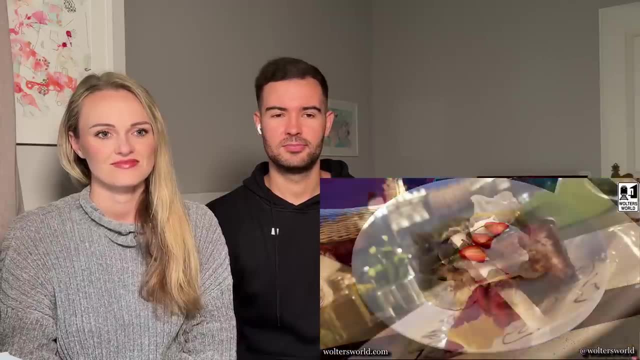 think you get a deep fried. well, i'd like to taste that. it's all the time with the, with the cabbage and the potatoes, again and again, and again. that's why yesterday i just got the cabbage rolls. i'm like, look, because then i know i'm gonna in the cabbage. 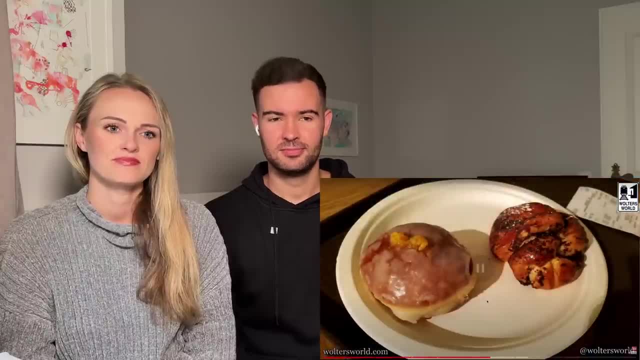 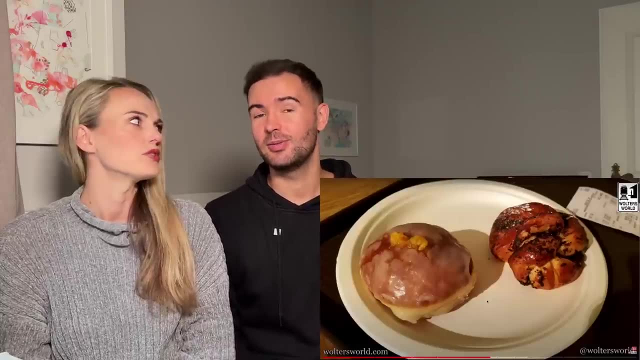 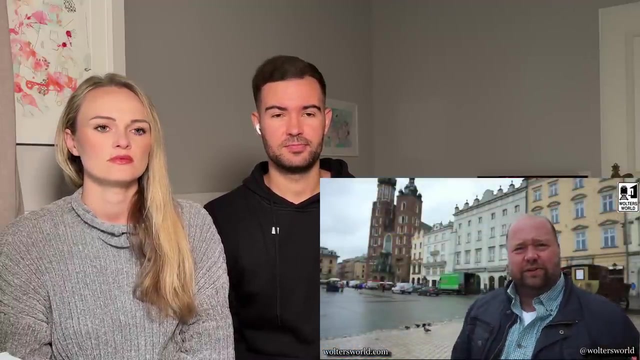 and it came with a side of mashed potatoes, and i just laughed. he said: try polish desserts. that's one thing that we didn't try when we were in poland. we had no, but we didn't have any desserts. okay, also kind of interesting: is they really love their tea here too? now the sixth thing. 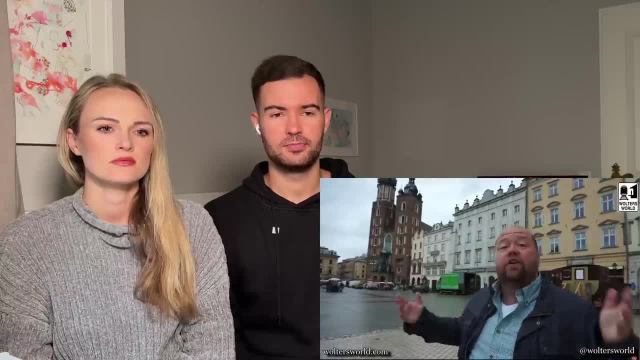 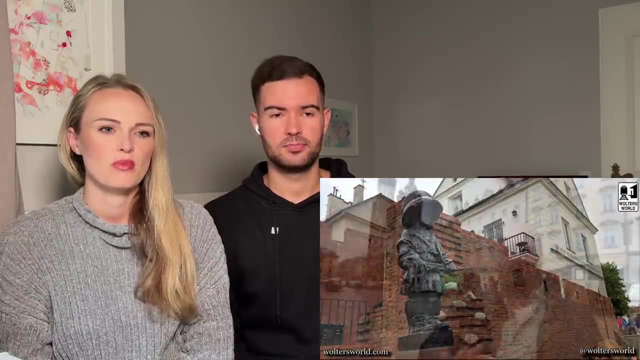 that might shock you as a tourist is you notice there's not very many tourists now. in krakow you do get about 10 million tourists a year. i mean, this is a very popular place because it's gorgeous, and i'll talk about that a little bit in a while, but i'm gonna start by saying that krakow is a 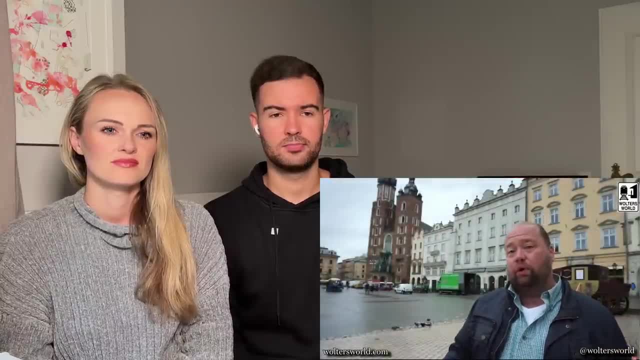 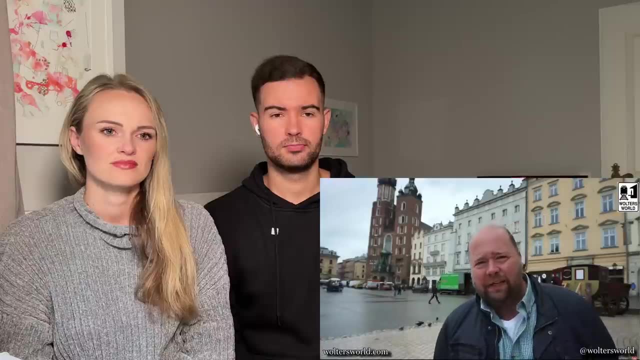 towards the end. but honestly, there's not a lot of tourists actually come to poland and so when you go around you really are kind of a special tourist because you're actually here, you might get people going. why are you lublin? yeah, why? why are you whoosh? why are you here? you know some places like. 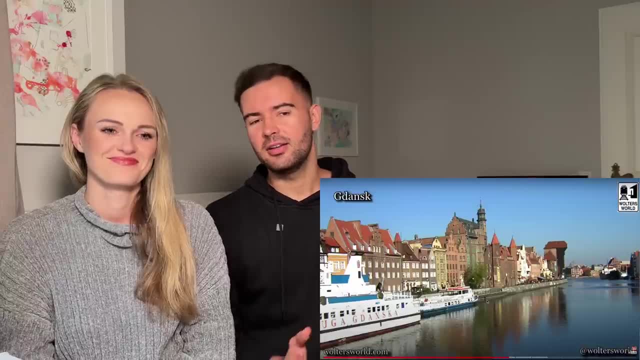 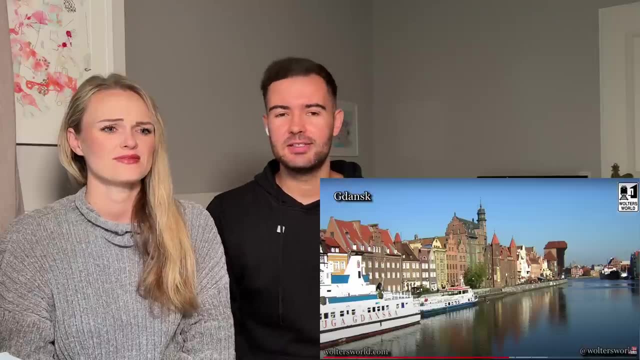 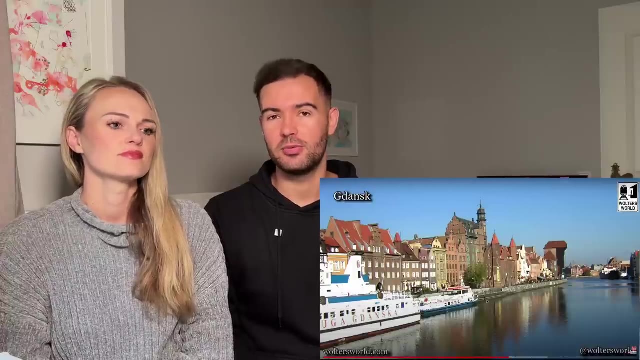 krakow. it's obvious, you know, but i don't know if it's like that nowadays, because a lot of people are visiting poland and i also can't think it is nice to have less touristy places, like we've been to a few places where it's just been so overwhelmingly packed with tourists that it 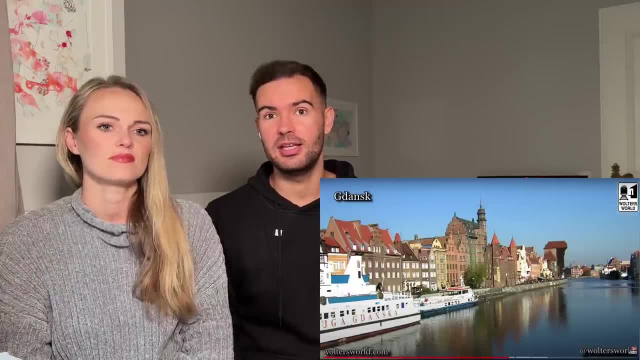 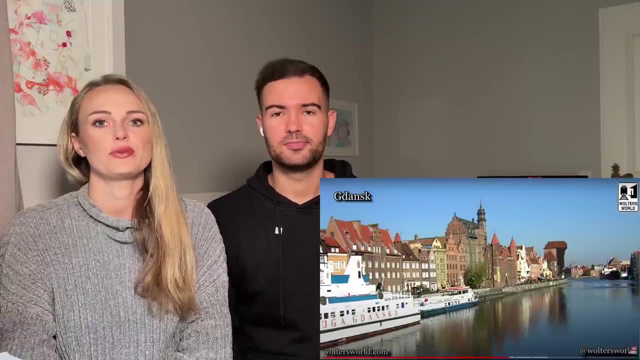 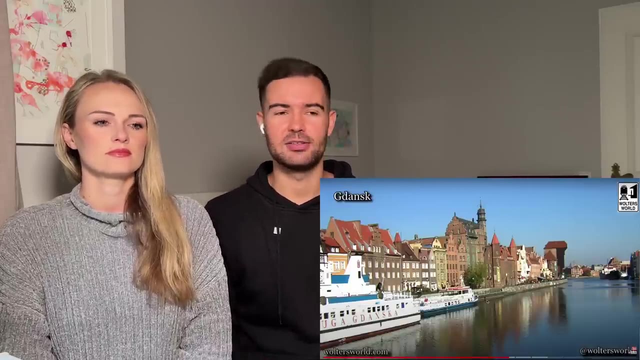 takes away from the enjoyment of the experience of being in that city or in that place. exactly every single tourist attraction is just too packed it's you can't even go view it. i don't like walking in crowded places, so for me, i mean, that's very nice about going to poland is the fact that 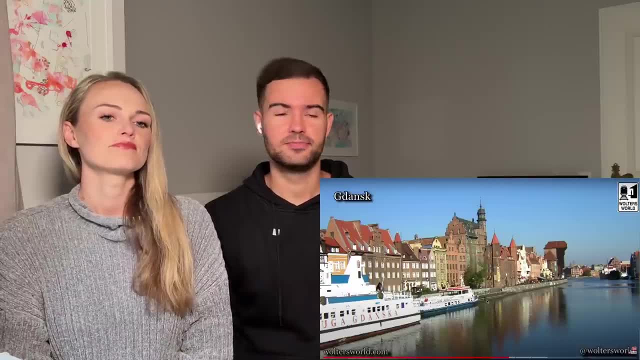 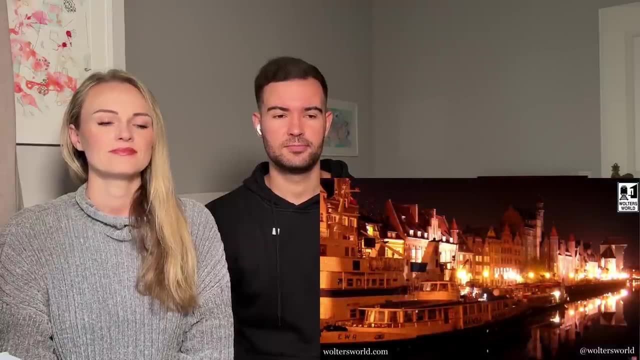 there's not as many people that are there now, but you go around and there's just so few tourists out there that you're like. you're like, hey, i'm going to go to poland, hey, i can kick back, relax and do okay. and what kind of leads on to that is? our next shock is: 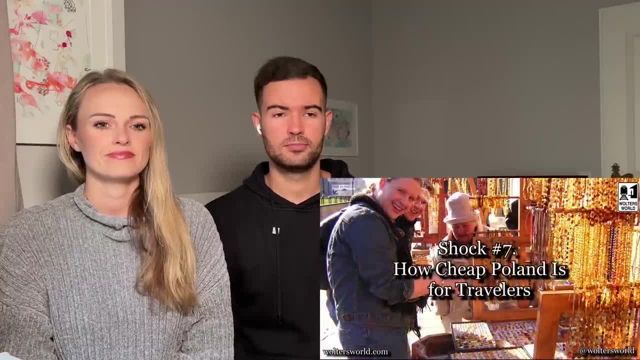 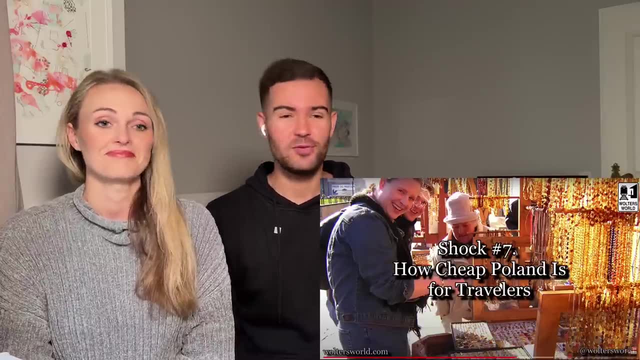 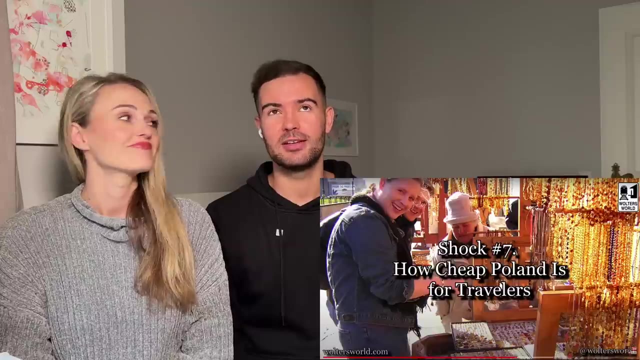 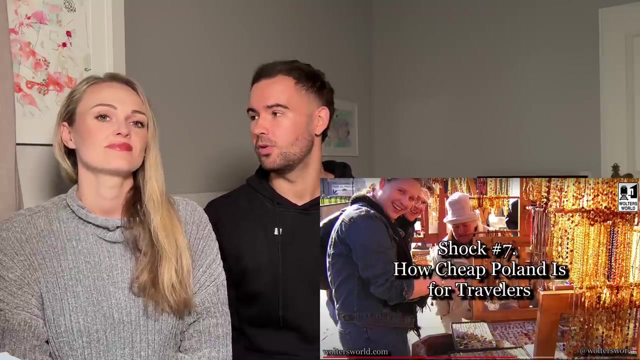 how cheap it is here because there's not a lot of tourists driving up the prices. yes, i can confirm that the food was like half the price compared to germany food and drink: yeah, it was really affordable. i think if you're earning a polish salary, maybe not as affordable, but for other europeans pretty affordable it's. it's nice because you can. 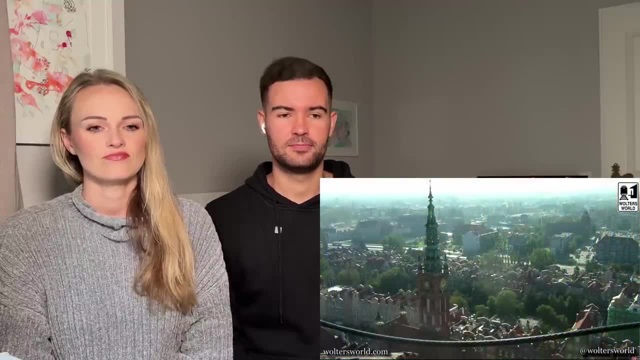 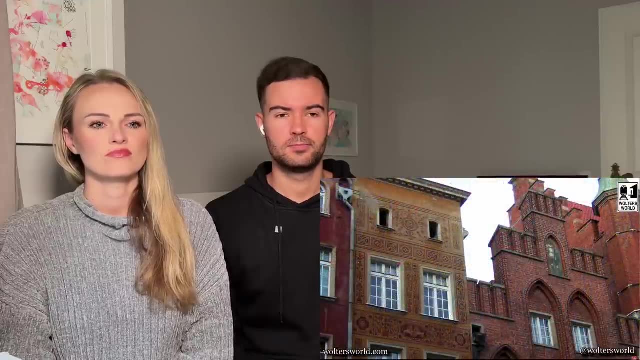 have a very affordable vacation here in poland: rooms, accommodation, food, drink, making merry, all kinds of stuff- and you'll see a lot of people come to like krakow or warsaw to come have a party weekend and stuff like that, because you really can. your money goes a lot farther here. 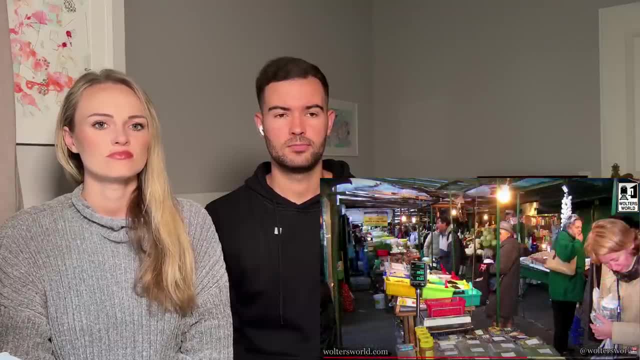 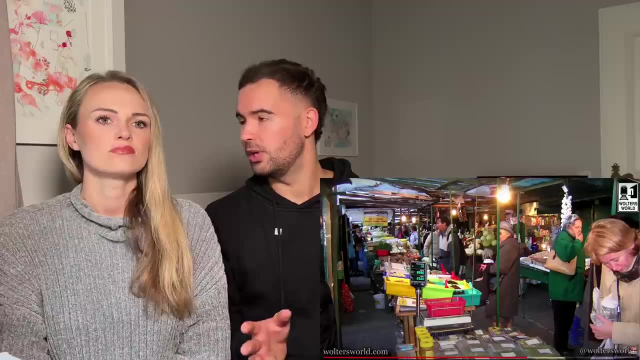 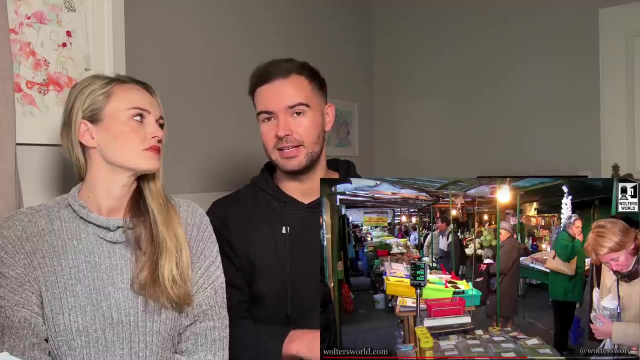 than other places, and that's what's really cool. now the next, and i agree with that because i've been looking at the past couple of weeks. i've been looking for places to stay in poland and comparing prices to other european cities like italy and the netherlands, and literally the price 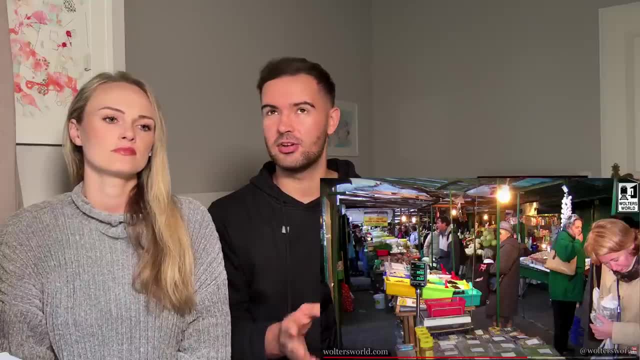 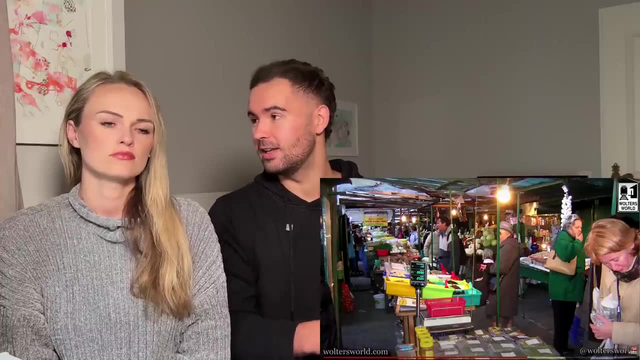 of what it would cost us to stay in- i think it's- krakow for four nights is the same price for one night in like a nice hotel in italy or in the netherlands. it's just 100 then tourist prices. it is, it's. 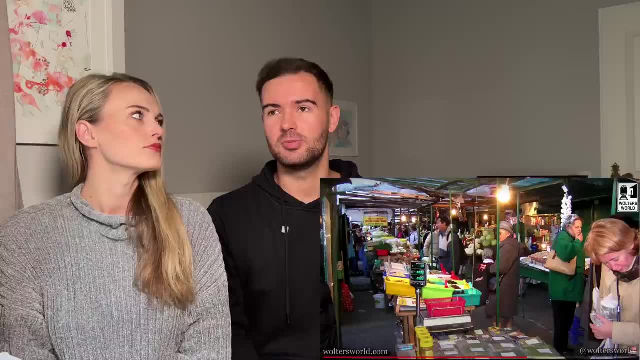 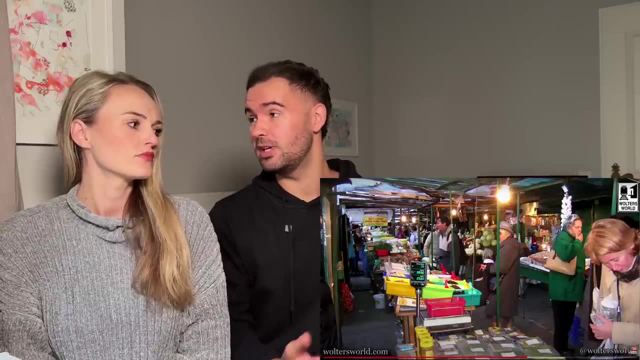 it's, it's tourist prices, like i mean, why would i go somewhere else where i'm only getting one night? but if i go to poland, i'm gonna have an equally as nice experience in terms of food and people and culture and things to see, and i'm gonna pay the same price, but i get four nights, exactly that's. 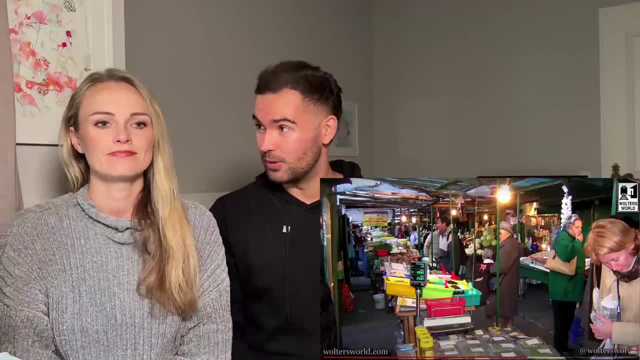 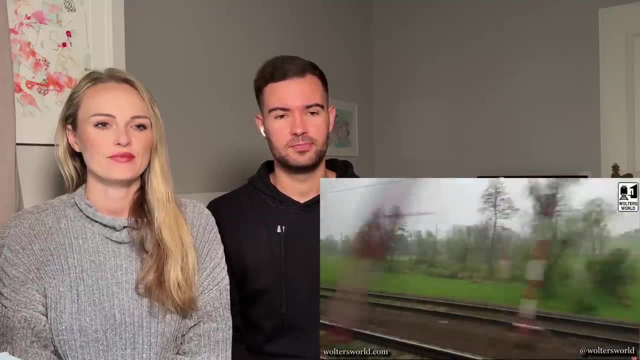 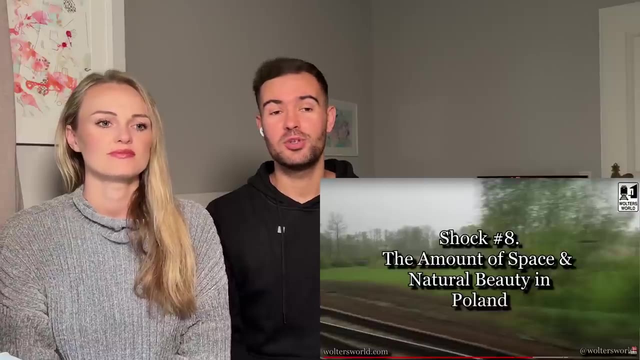 why we're going to poland. that's why we're going to poland as well. it's affordable. the next thing is the amount of natural beauty and space in poland. look, yeah, this is a huge country. it's one of the biggest countries. that is what we're. that is what we're looking forward to. i'm looking forward. 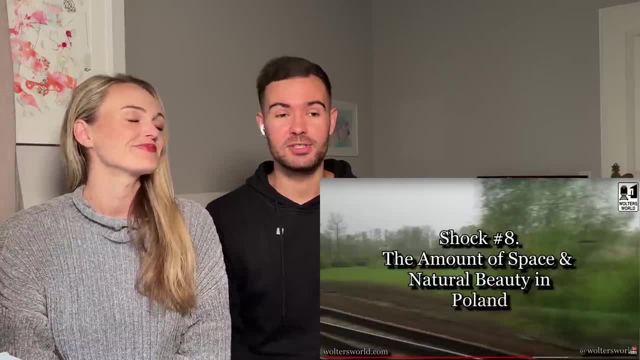 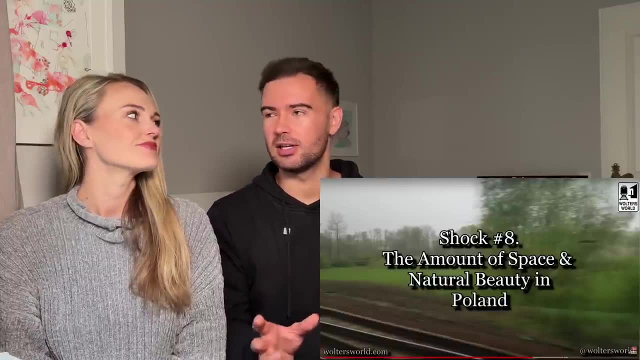 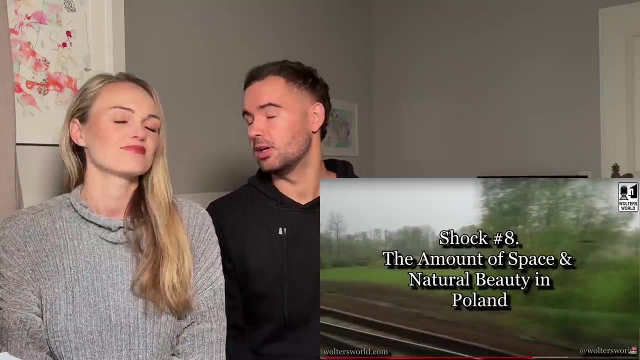 to the train rides, can you imagine going through some beautiful scenic militants? i don't know what good train rides are, probably very scenic, going through poland like. i'd love to know maybe which ones to book, which ones are between various cities, like the most popular? that would be nice to know. 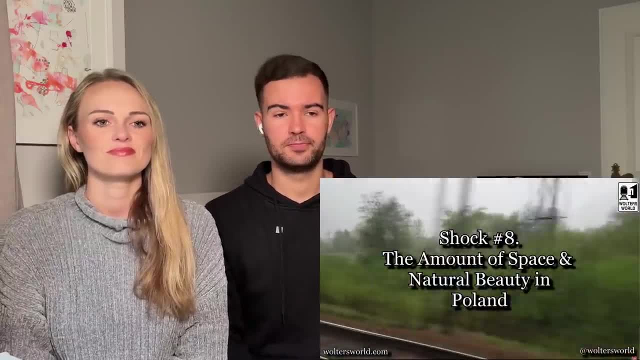 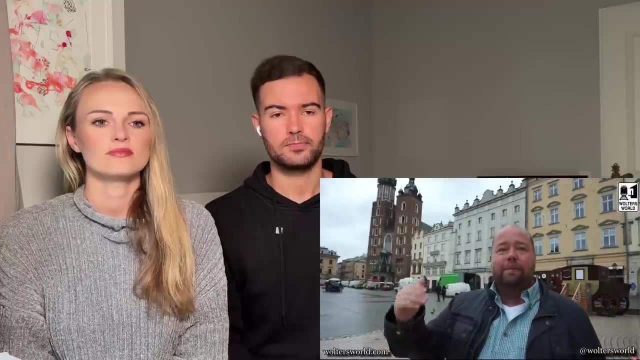 countries in europe and the thing is you're going to be going between these different towns, whether it's on a bus or a train, things like that- not super fast, but it's going to be a lot of fun. trains, but fast enough trains and you're going around and it's just amazing how big the country. 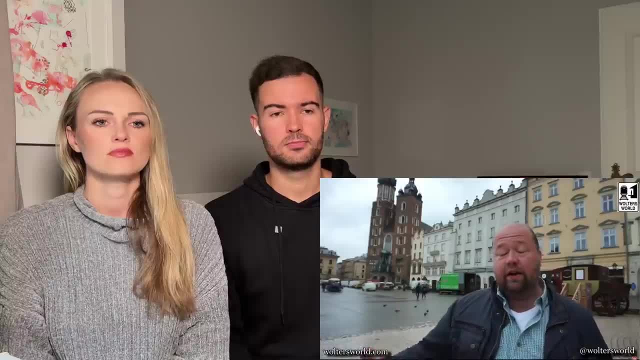 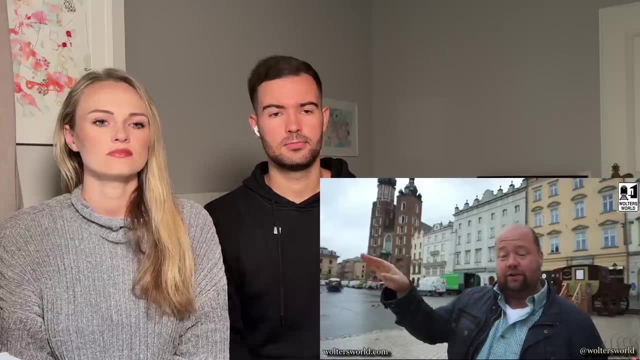 is, but also the natural beauty you see when you go through there. and what's nice is when you go through and you can go. if you're in the north, you're going to gdansk and hey, well, that's one of my favorite. krakow and gdansk are my two favorites. you're up in gdansk, you come down a. 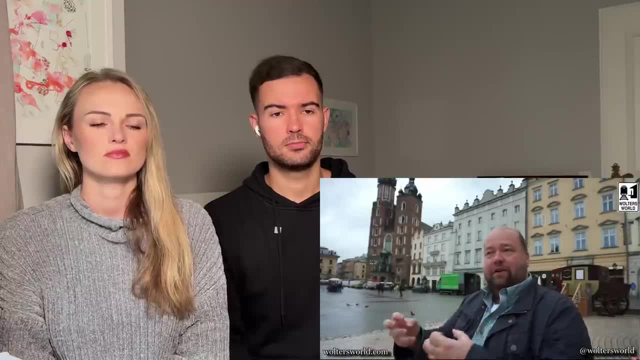 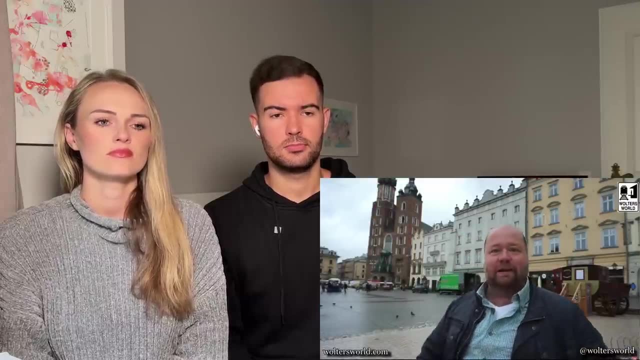 bit. you can go over to the missourian lakes and see the the castle that's right by there, the marlborough castle, which is on the way towards there. go to the lakes and enjoy that. go to the coast in the north, in the south you've got the tatras mountains and you go to zakopane. 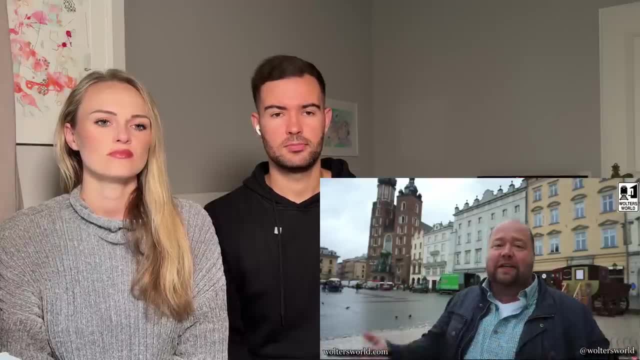 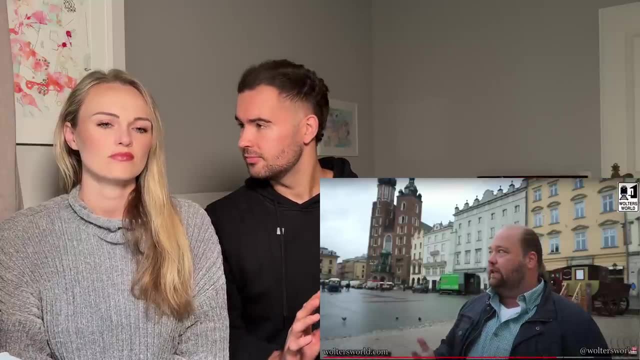 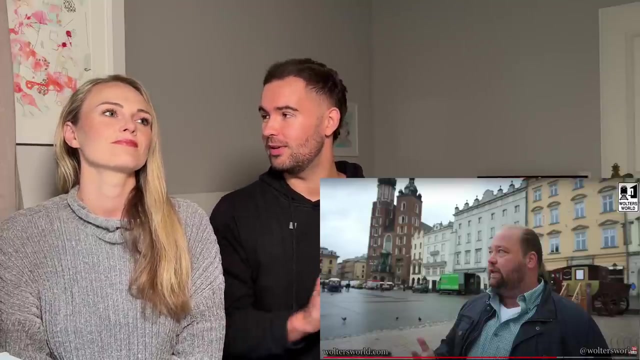 stay there. tons of europeans go there to ski in the winter because, yes, it's beautiful and it's cheap. remember what i said before. but you have this natural beauty like, wow, this really is the extensive beauty of poland and the centricity of europe, and the fact that it's cheap. 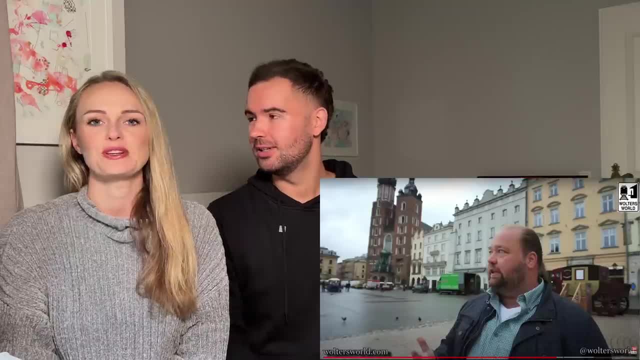 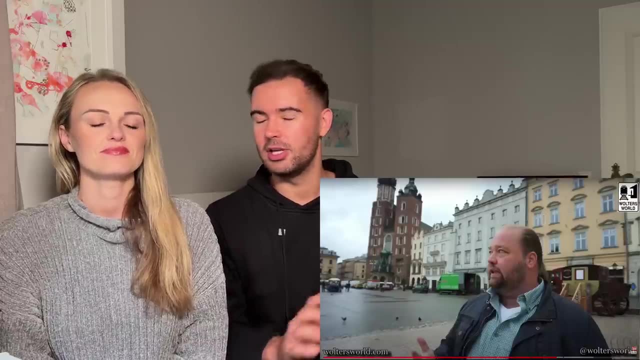 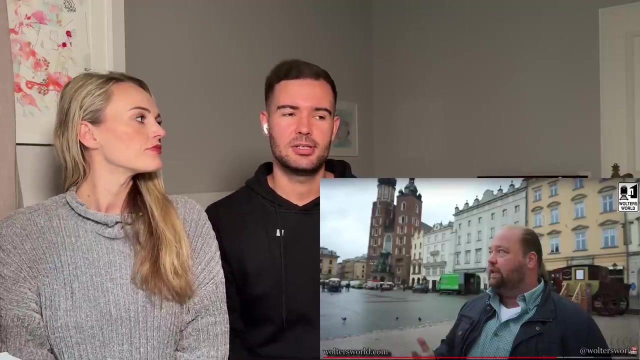 it's like all in one, absolutely, like literally. we had- i was speaking to someone that did some skiing earlier on in the year and they were in poland well skiing. i think it's the. i don't know he said the word now, but it's the- 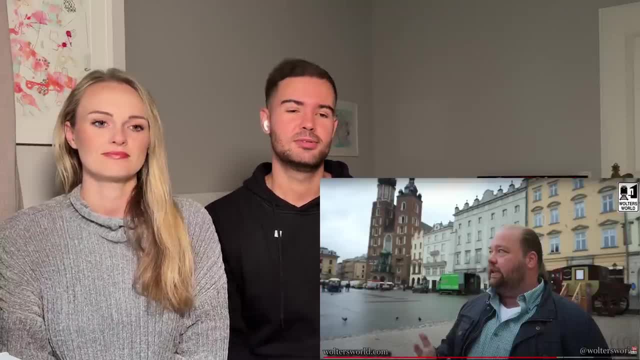 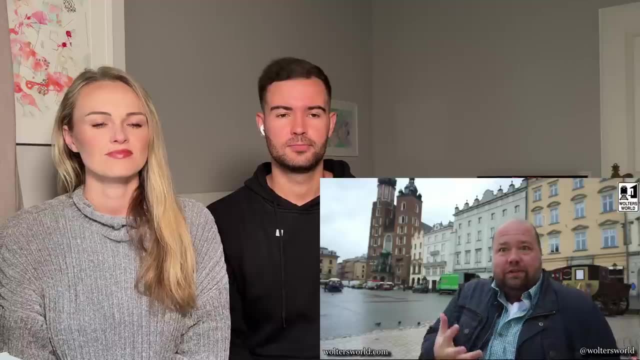 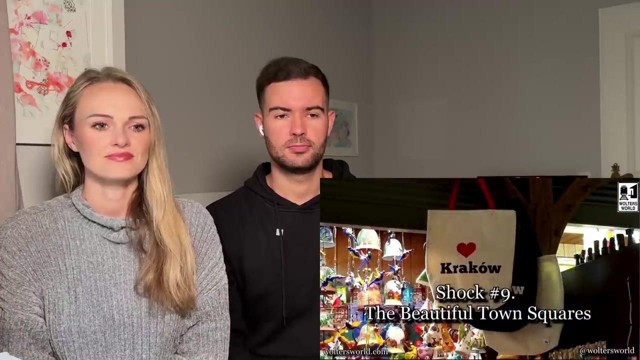 mountains in the south. so zakopane, zakopane is. i understand why they have. all their tourism propaganda is about, you know, the natural beauty of poland, because it really is beautiful. having said that, the next thing that'll shock you is how amazing the town squares are here in poland. 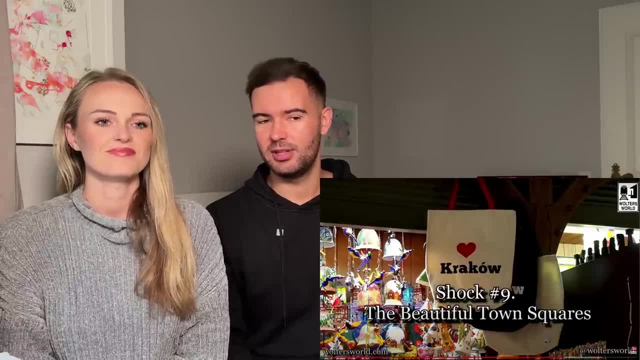 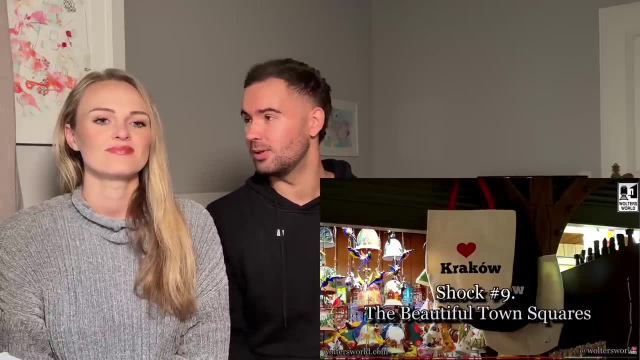 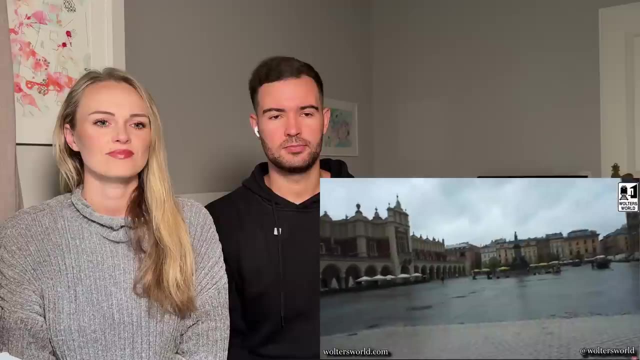 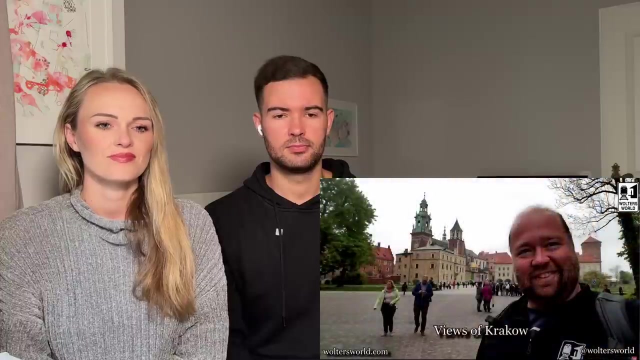 so old town squares is probably the best well-preserved areas in the cities, probably the most expensive as well, probably because that's where the tourists are. but yes, here in krakow you've got the, the cloth hall over here to check out. you've got the saint mary's church over there. you've got all these things. i'm sorry. 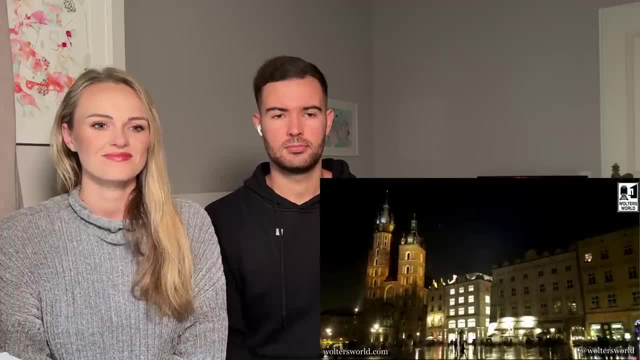 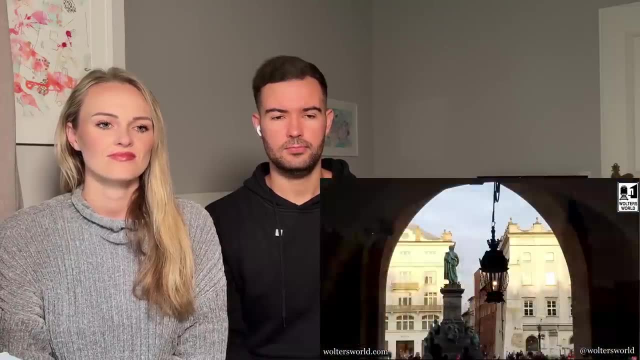 you've got all these things to go and see and this is actually the largest town square in the european in europe and it's amazing. but it's not just here. you go to warsaw to see their old town square. they really built from scratch vraklav. go see the old town of lublin. 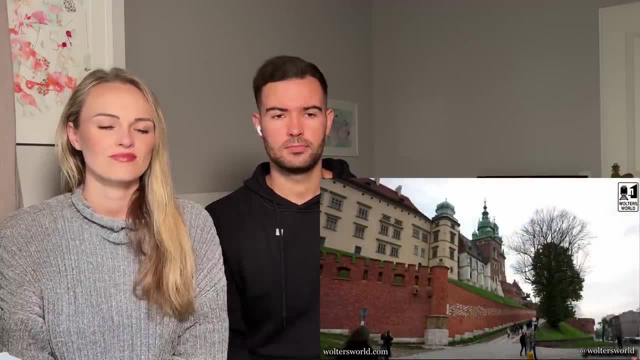 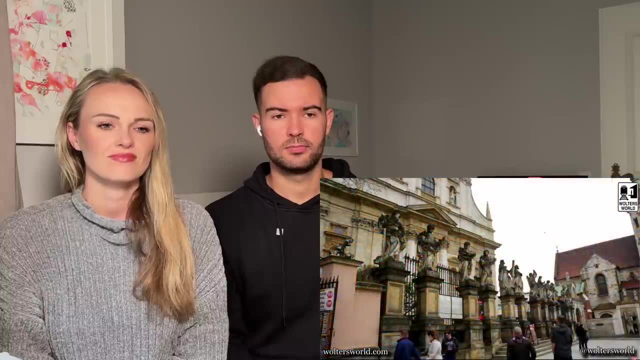 oh, man, godan's the port city of get honest. man, you just walk around there. see the neptune statue. you're like man, this is so cool. and you have all these beautiful squares. you have all these beautiful buildings that have been rebuilt after the war- or maybe they're still there from before. 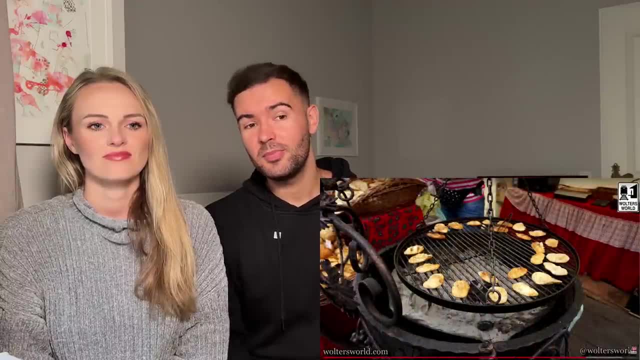 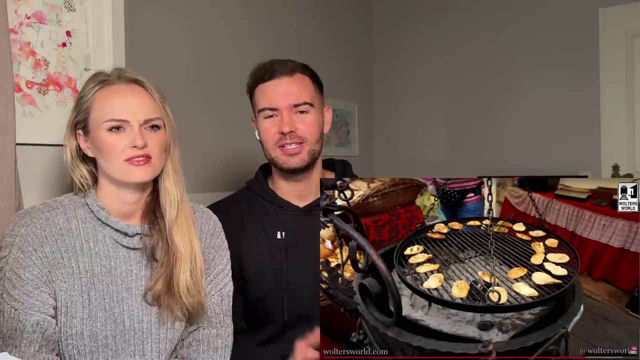 the war. you have that beauty that looks like pierogi on coals. what's bread? i don't know. it does not look like pierogi. what is that is it looks like… looks like bread. let us know in the comments down below. beauty that are not a lot of people think of. 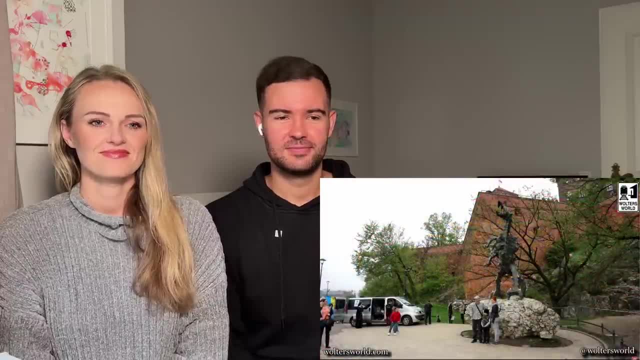 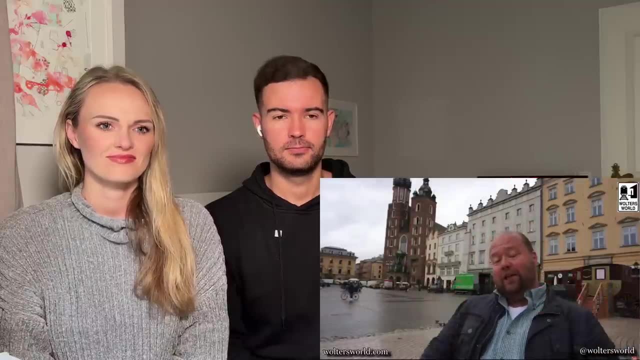 because when they think of poland, you're thinking of you know, oh, it's just, it's farmland and stuff like that, and look, there are some just amazing places here in poland, so it's definitely worth checking out. and the tenth thing that might shock you when you do come to poland is the 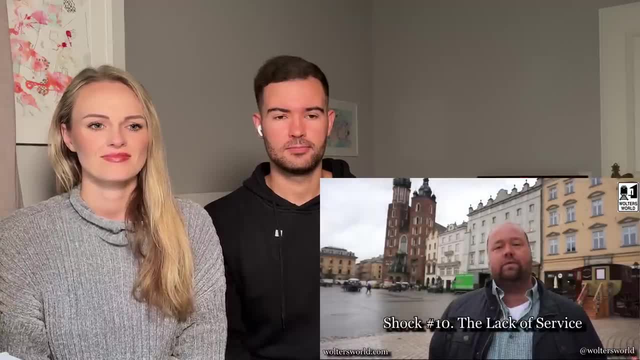 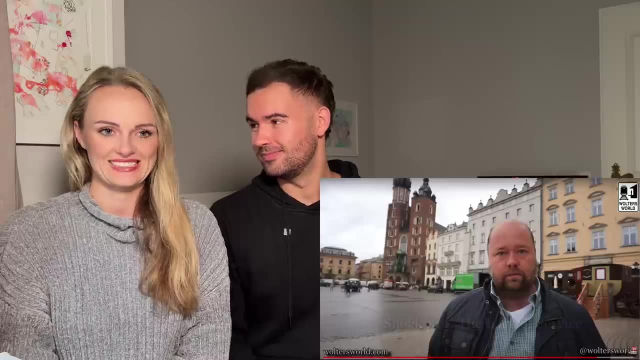 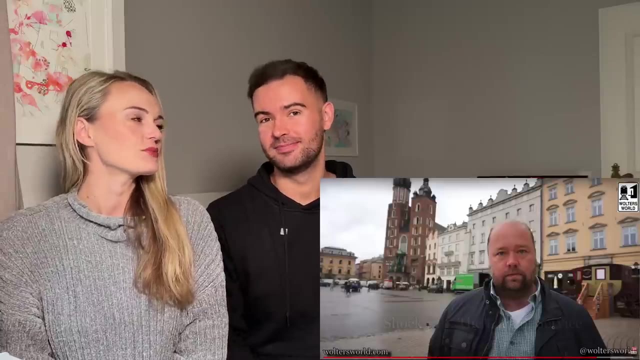 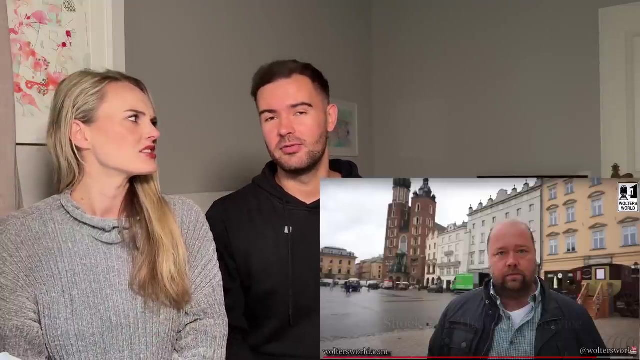 lack of service. so remember that polish face. this is your service. that is europe in general. yeah, you just don't get service at restaurants or good service. we're spoiled from south africa. yeah, it's mostly self-service here, like you go and order at the front and then when it's ready, you go fetch it, unless you're sitting in a very classy fancy.